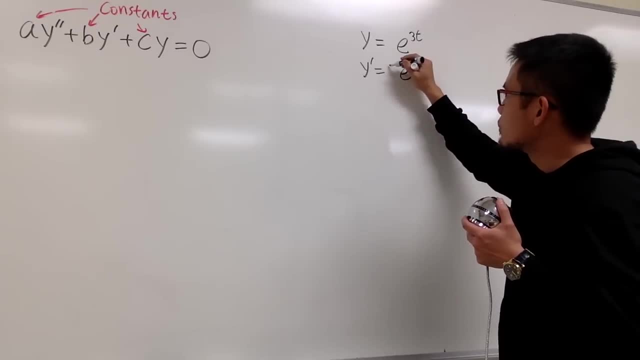 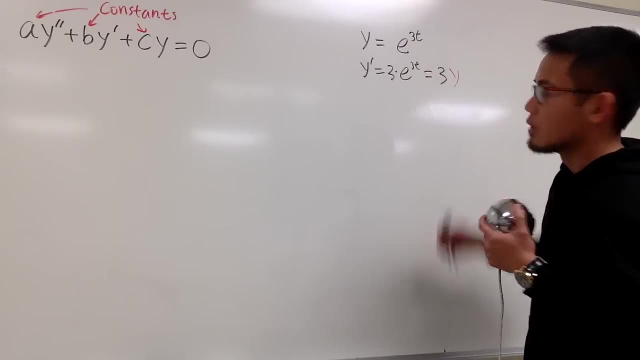 But the chain rule says I will have to multiply by 3, right? So let me put it down right here. right, And you see, these three stays, and this is just the original. So 3 times y, right, And likewise I can do it again. 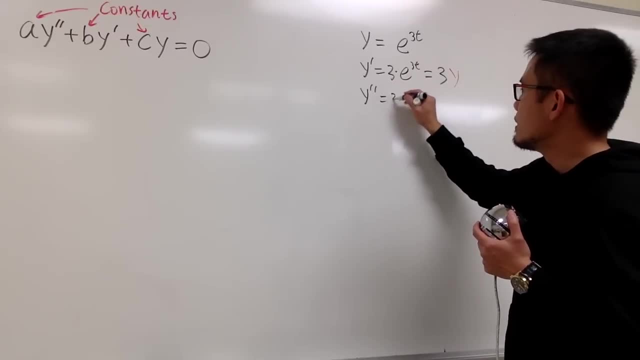 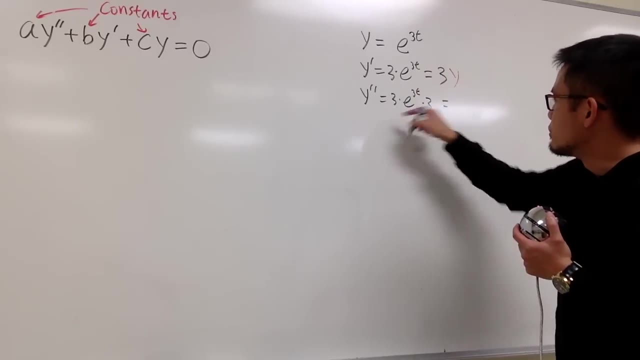 y, double prime it's going to be. We will keep this 3 times e to the 3t, but then we multiply this 3, right for the derivative by the chain rule. 3 times 3 is 9, and e to the 3t is the original. 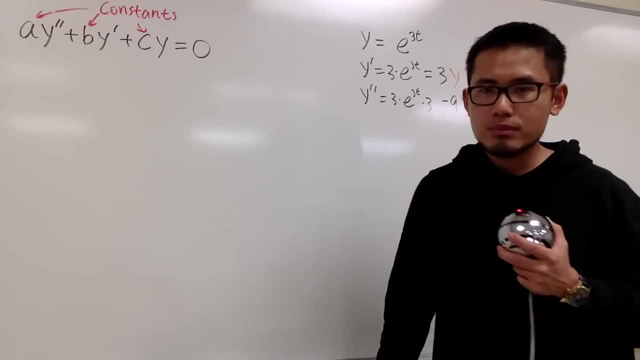 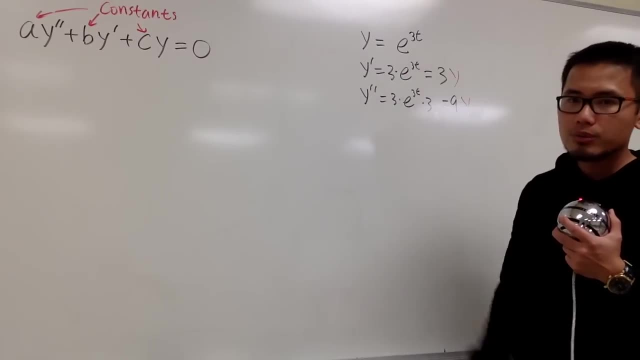 And you see, whenever you have an e to the some power, the first derivative, the second derivative, they are just going to be the constant multiple of the original right. So what this is telling me is that this will suggest. Let me just put this down. 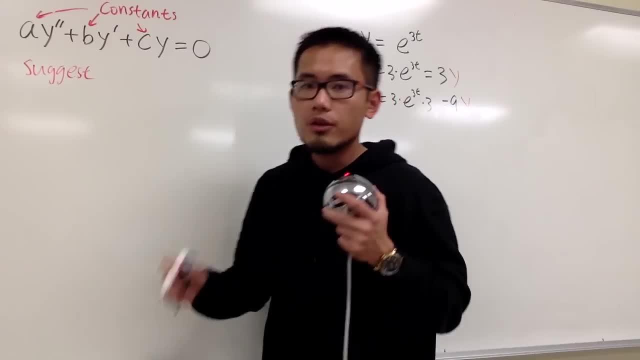 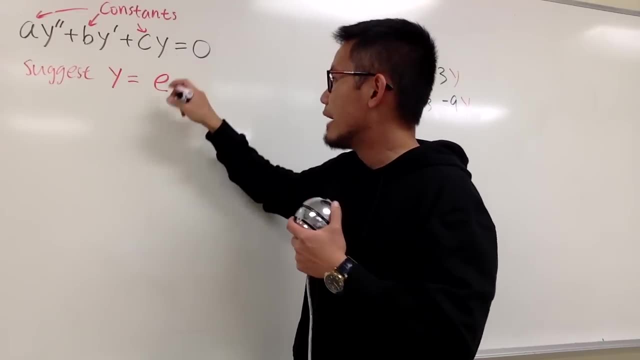 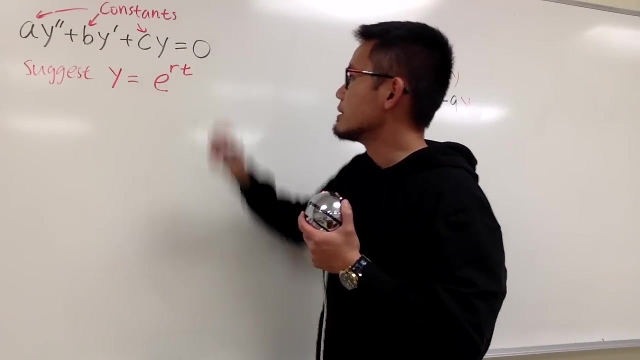 This suggests? It suggests that for the function we should have the form y equals to e, to some power times t. I don't know what this number should be Earlier, I just used 3, right? So in general let me put down r times t. 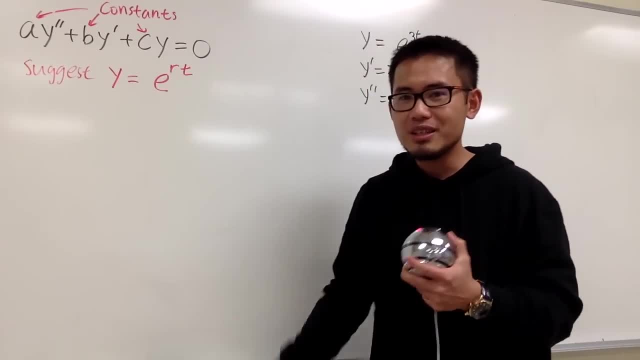 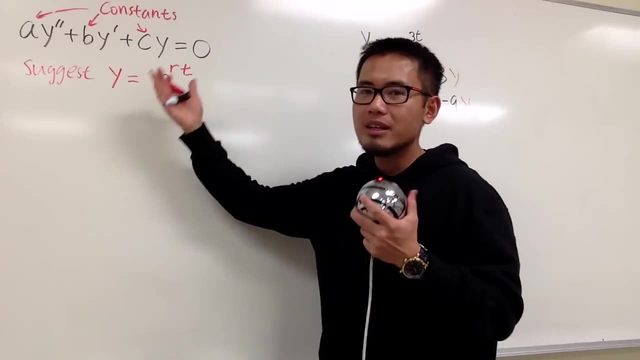 And, once again, for the second-order situation, we usually use t because there are a lot of applications that enforce time and things like that. Anyways, this is my starting. First of all, we begin by saying y is equal to e, to the rt power. 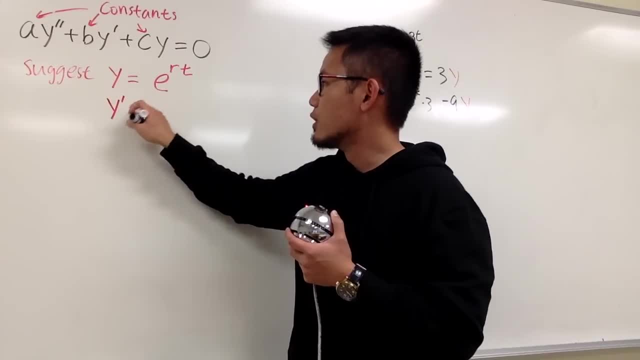 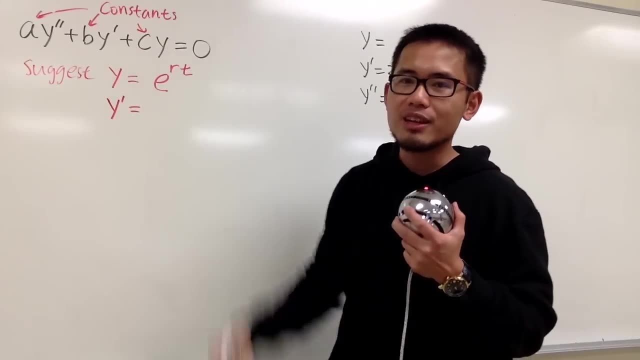 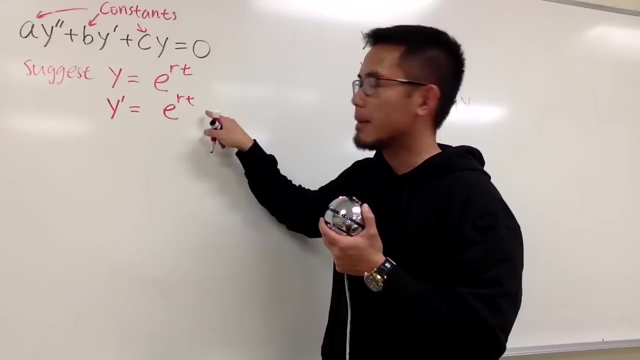 And the idea is that I'm just going to go ahead, differentiate this twice and then plug in. Hopefully we can squeeze out some conditions that will help us to solve for this kind of differential equation. All right, y prime is going to be e to the rt times r. 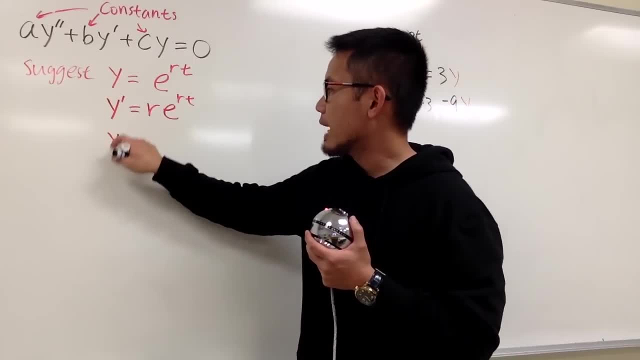 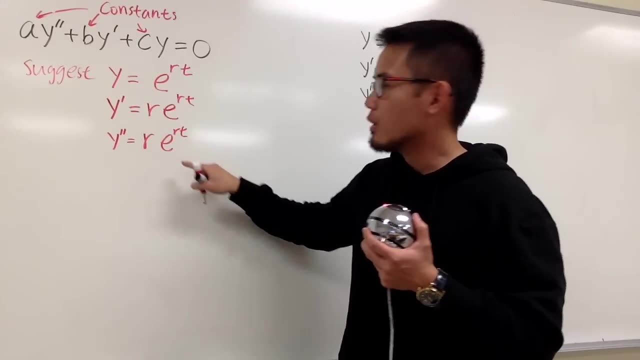 Let me just put r in the front And then y double prime is going to be this: right here repeats: right r e, r t. But then we multiply by another r, which will be r times r, which is r squared. 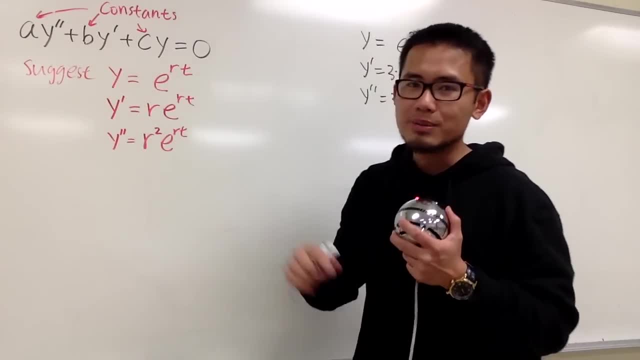 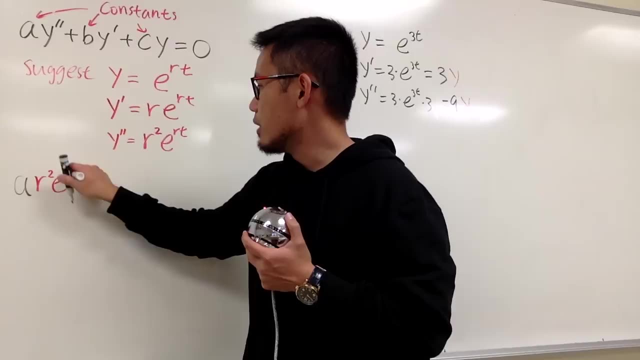 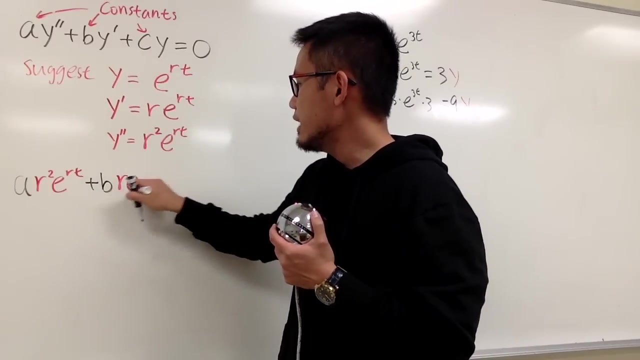 And now let me put all this into there. correspondingly, Here we have a: y double prime is r squared e to the rt, And then we add it with b, so we put on plus b: y prime is r, e to the rt. 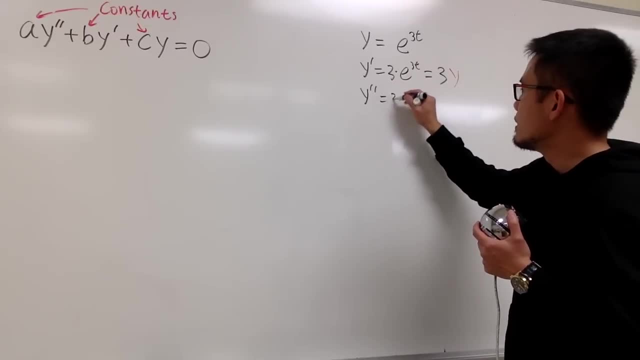 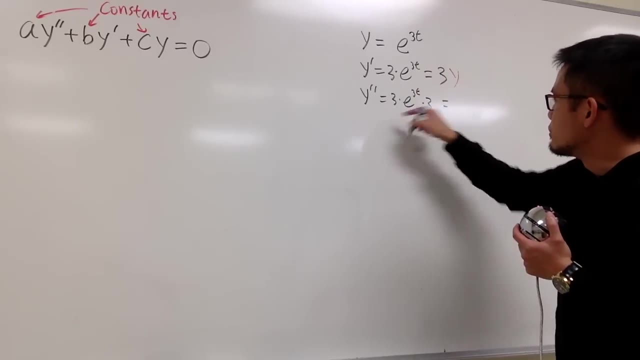 y, double prime it's going to be. We will keep this 3 times e to the 3t, but then we multiply this 3, right for the derivative by the chain rule. 3 times 3 is 9, and e to the 3t is the original. 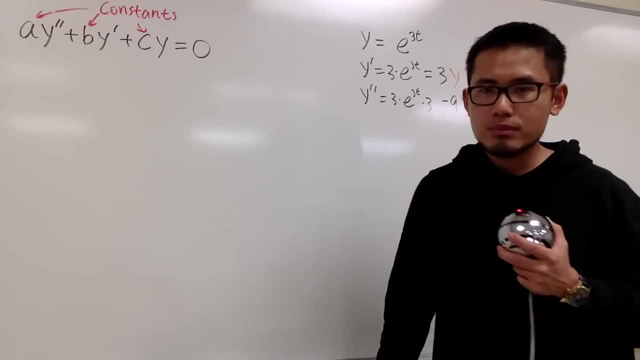 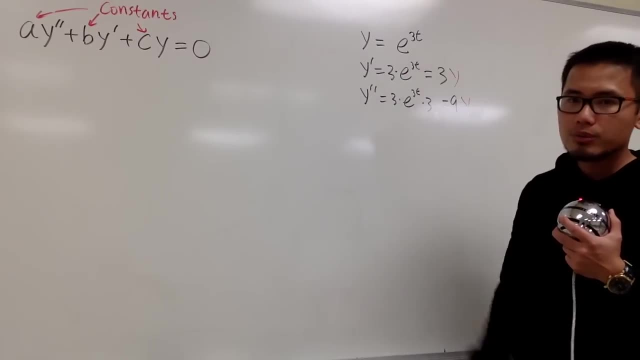 And you see, whenever you have an e to the some power, the first derivative, the second derivative, they are just going to be the constant multiple of the original right. So what this is telling me is that this will suggest. Let me just put this down. 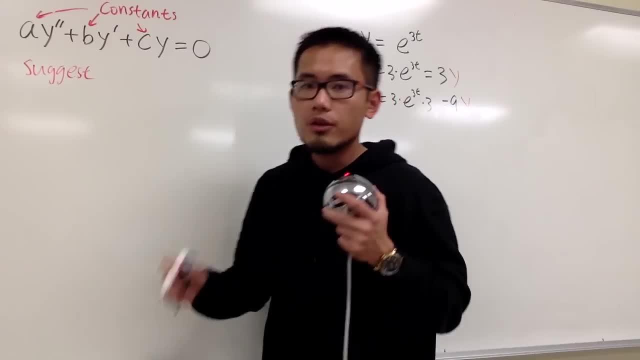 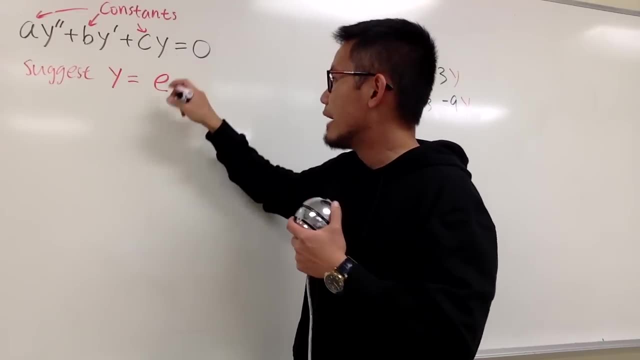 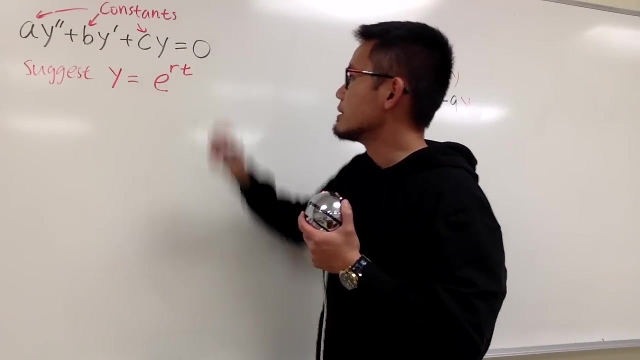 This suggests? It suggests that for the function we should have the form y equals to e, to some power times t. I don't know what this number should be Earlier, I just used 3, right? So in general let me put down r times t. 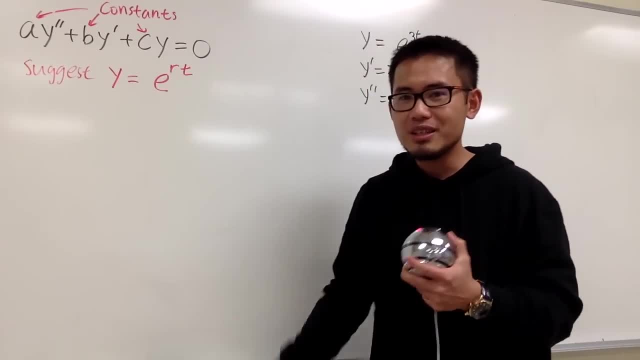 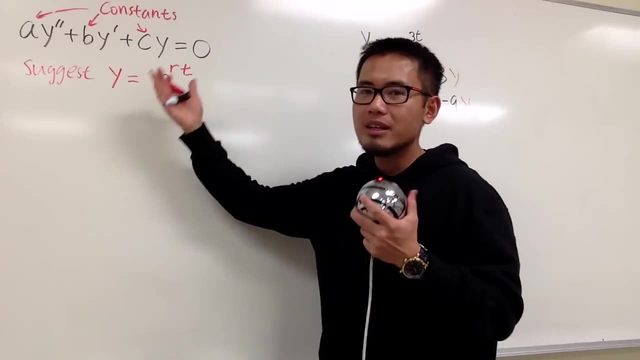 And, once again, for the second-order situation, we usually use t because there are a lot of applications that enforce time and things like that. Anyways, this is my starting. First of all, we begin by saying y is equal to e, to the rt power. 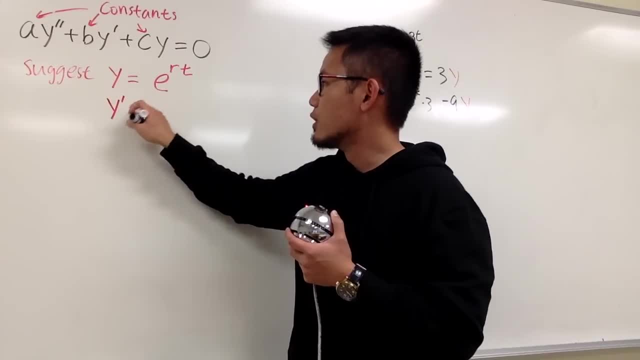 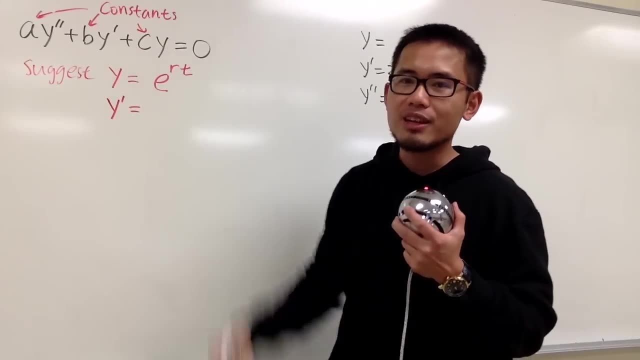 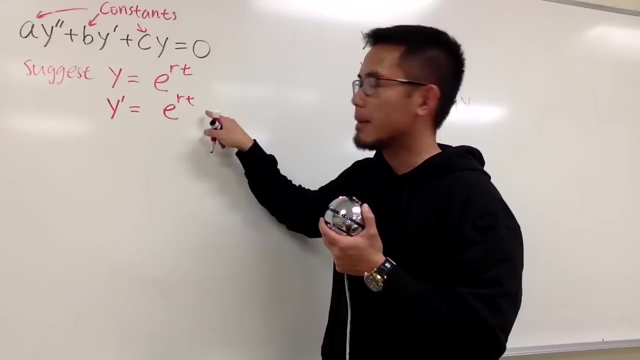 And the idea is that I'm just going to go ahead, differentiate this twice and then plug in. Hopefully we can squeeze out some conditions that will help us to solve for this kind of differential equation. All right, y prime is going to be e to the rt times r. 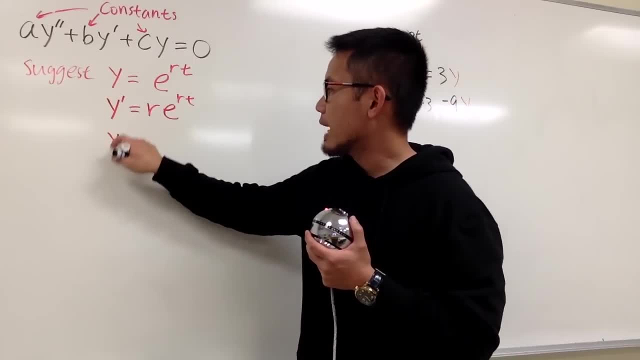 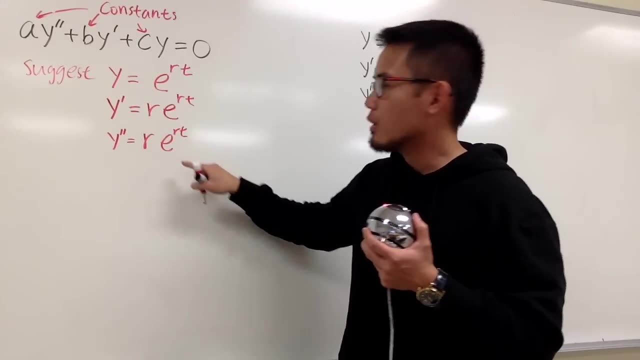 Let me just put r in the front And then y double prime is going to be this: right here repeats: right r e, r t. But then we multiply by another r, which will be r times r, which is r squared. 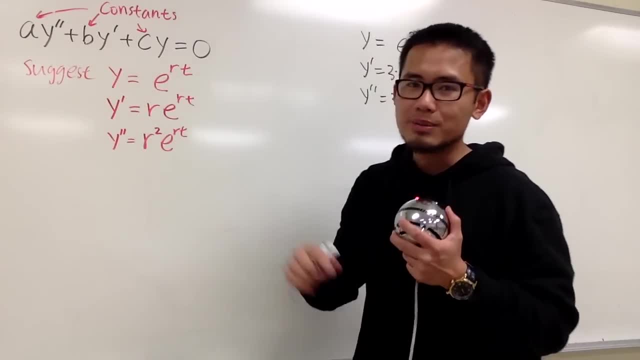 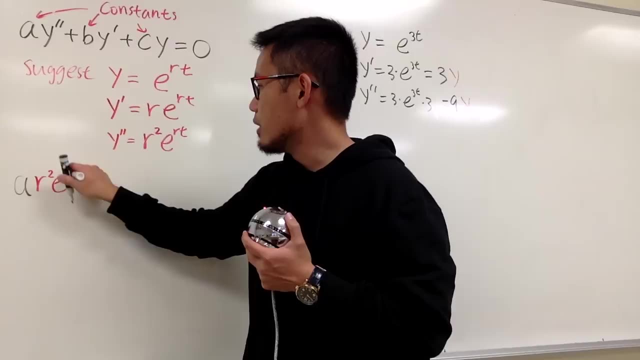 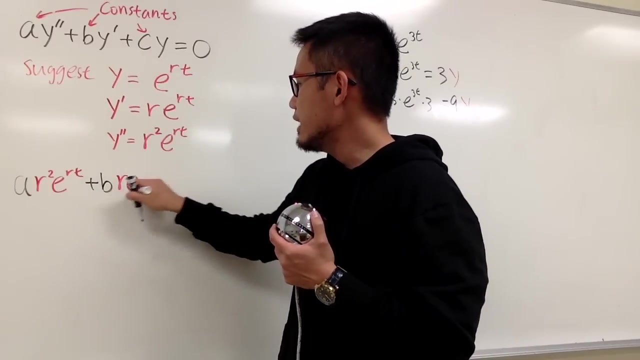 And now let me put all this into there. correspondingly, Here we have a: y double prime is r squared e to the rt, And then we add it with b, so we put on plus b: y prime is r, e to the rt. 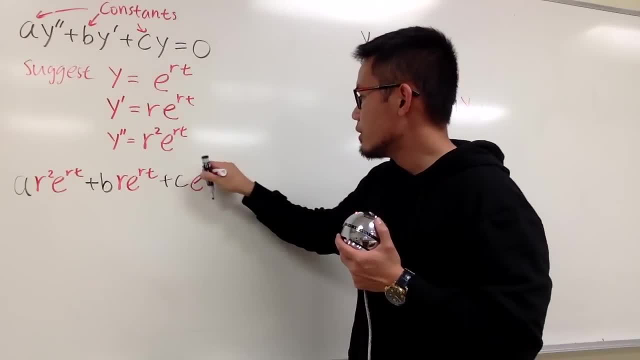 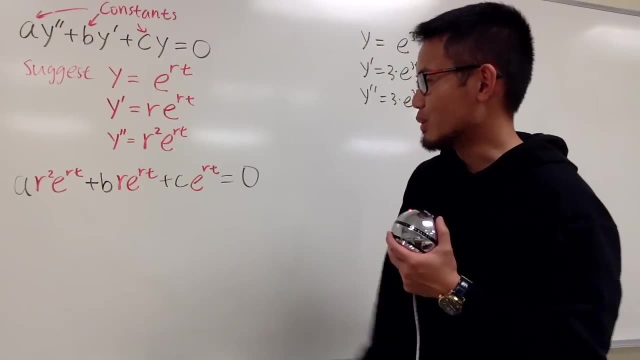 And then we continue. plus c, y is e to the rt, And this right here is equal to zero. And now can we kind of squeeze out a condition. Let's see what can we do. Every term has e to the rt, so we can factor it in, of course, right. 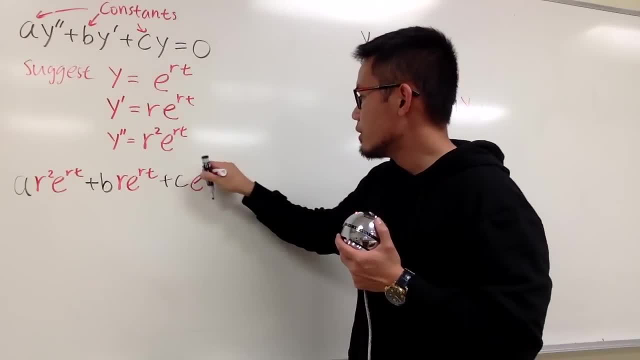 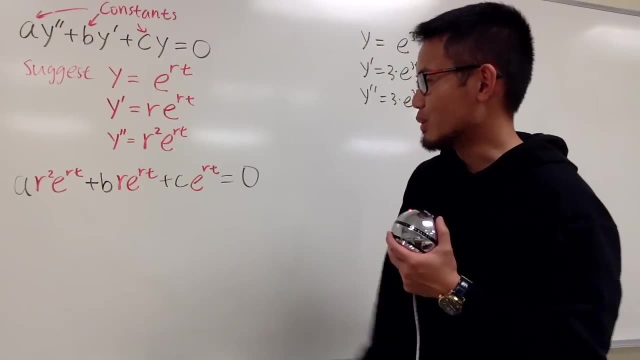 And then we continue. plus c, y is e to the rt, And this right here is equal to zero. And now can we kind of squeeze out a condition. Let's see what can we do. Every term has e to the rt, so we can factor it in, of course, right. 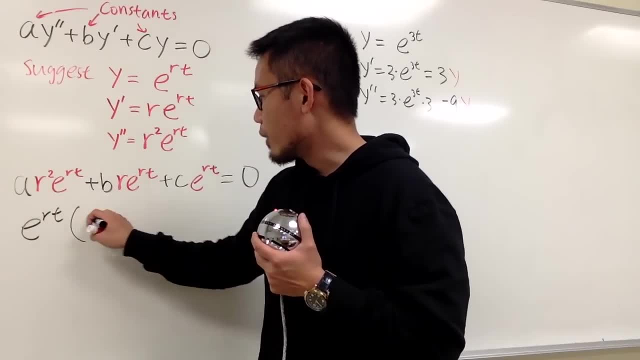 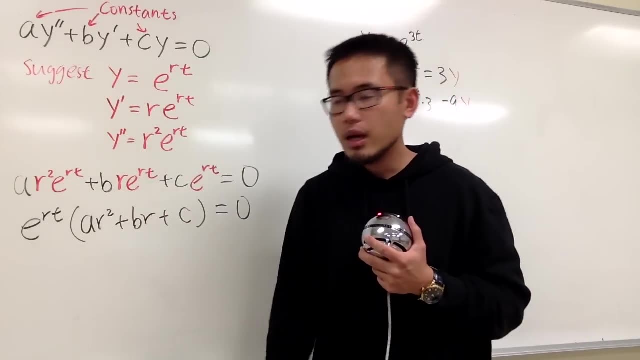 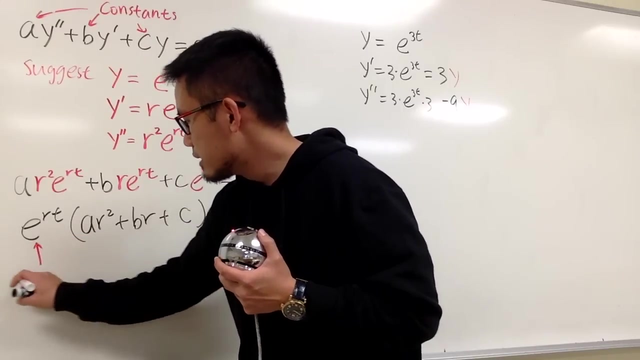 e to the rt, And that will give us: ar squared plus br plus c equals to zero. All right, this is an exponential part right. Exponential function e to the, something This right here we know is negative, Never zero, isn't it? 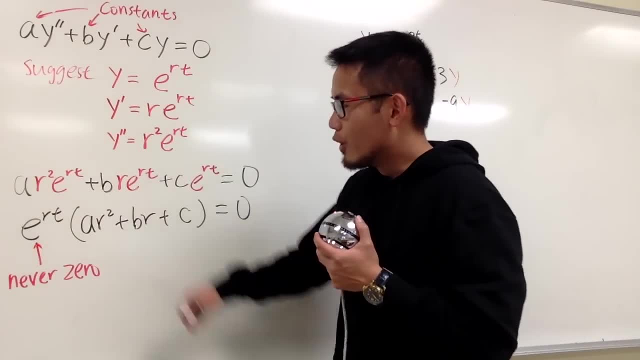 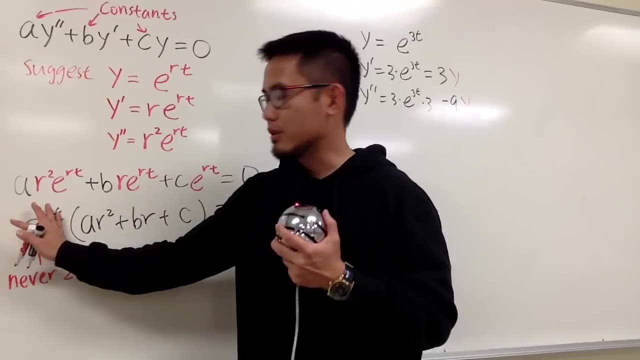 Never zero. let me just spell it out much better. So when we have this quantity, times that quantity, since e to the rt- is never zero. so you can either divide it out or you can just forget about it, because we just want to focus on this. 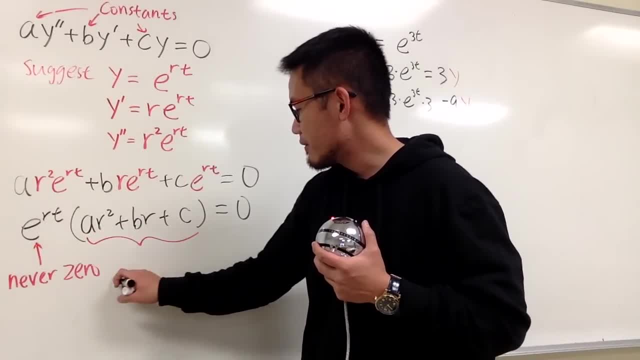 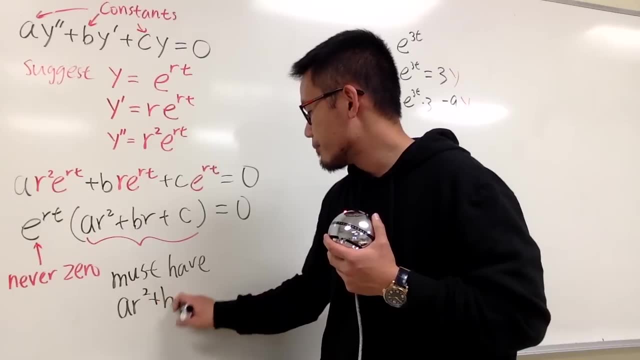 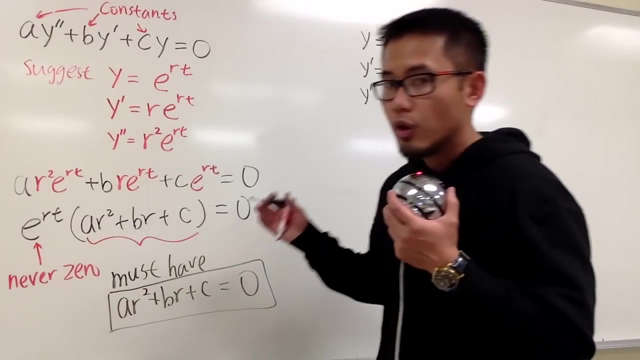 So that means we must have this part. We must have- let me just write it down- We must have the situation that ar squared plus br plus c, equal to zero. In fact, this, right here, is the condition that we need, Because from here this is pretty much just a quadratic equation, isn't it? 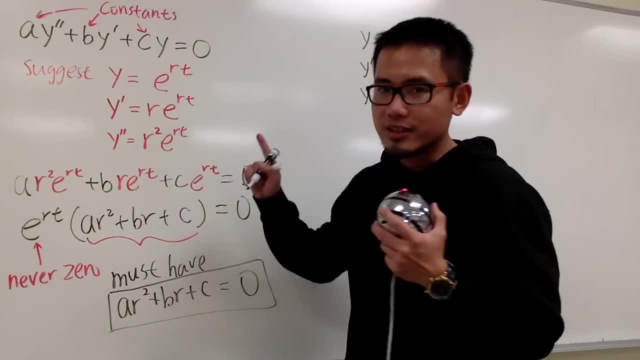 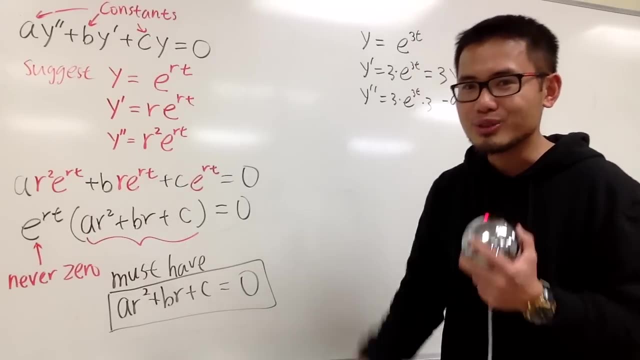 Quadratic equation in terms of r. From here we can solve for r and we can just plug it into the r here and we can generate the building blocks of this solution. And I'll show you guys what I mean by that. 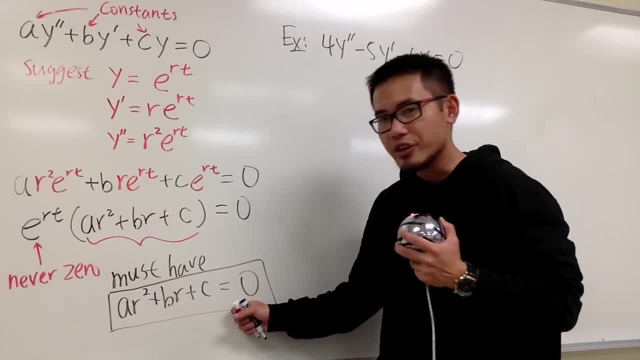 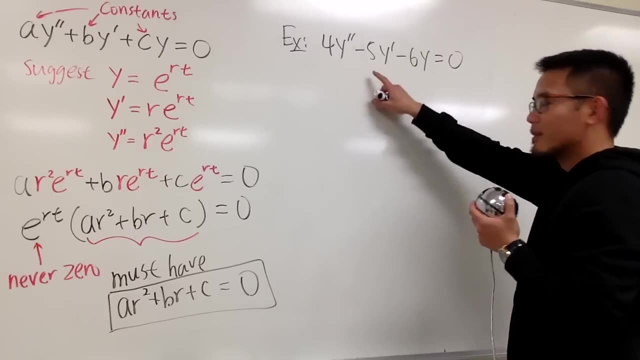 And before I show you guys an example, let me tell you guys that this equation here has a name. This is called the characteristic equation and this is also called the acceleration equation. And now let's go ahead and solve this, For y double prime minus 5y. prime minus 6y is equal to zero. 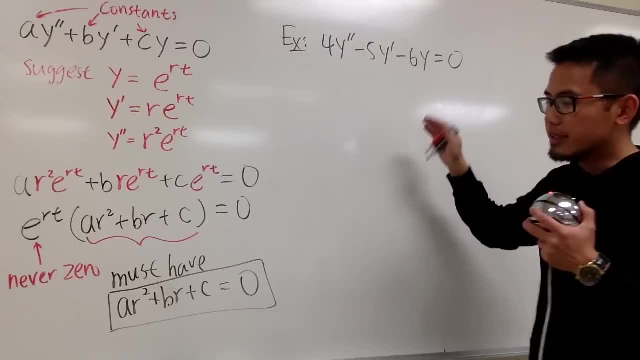 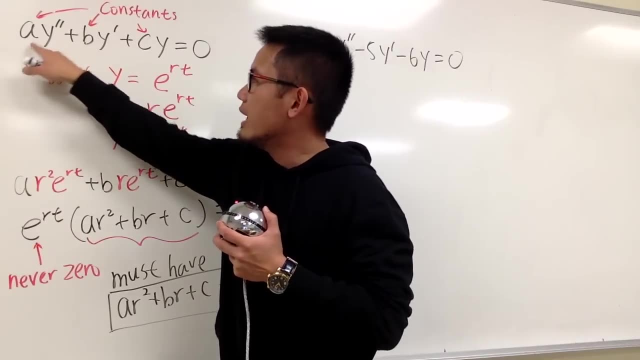 The first step is we have to take this and change it to its corresponding characteristic equation And check this out Earlier, when we started with ay double prime, we will end up ar squared right. So y double prime corresponds to r squared. 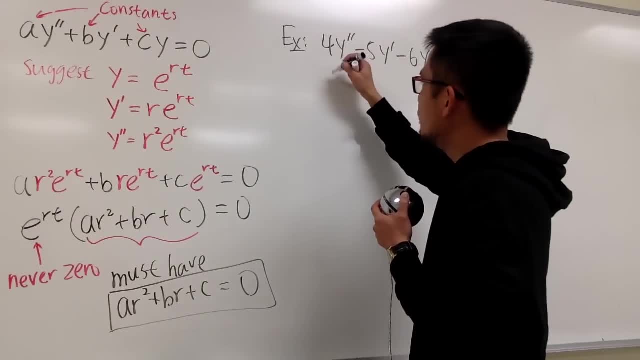 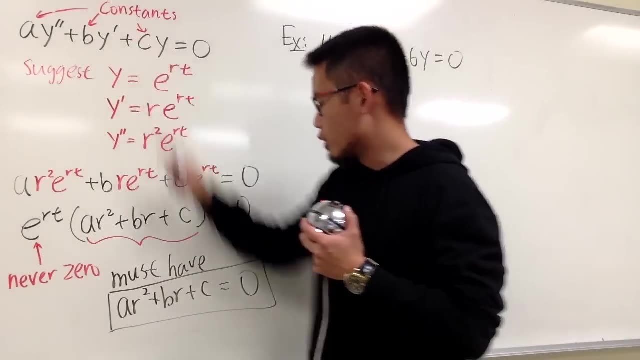 That means right here. the first term is going to give me 4.. So that's going to give me r squared. And then we just continue Minus 5, and the y prime corresponds with r. We change that to r, right here. 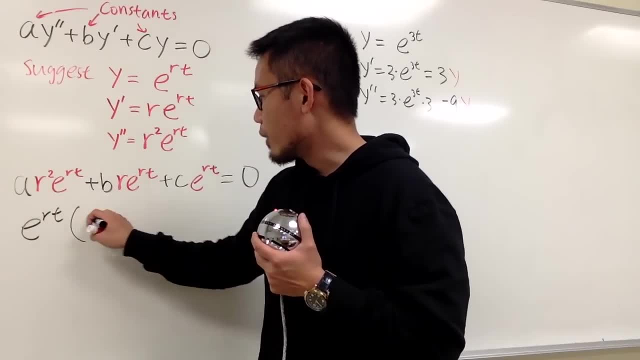 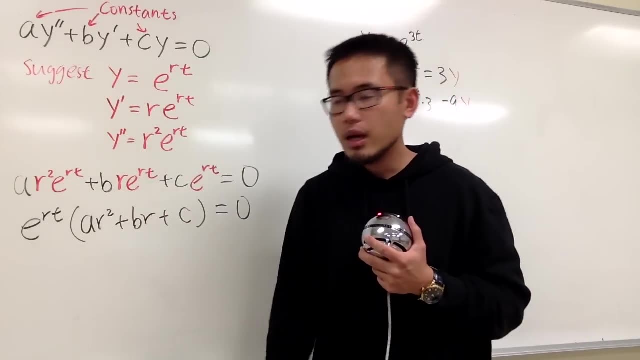 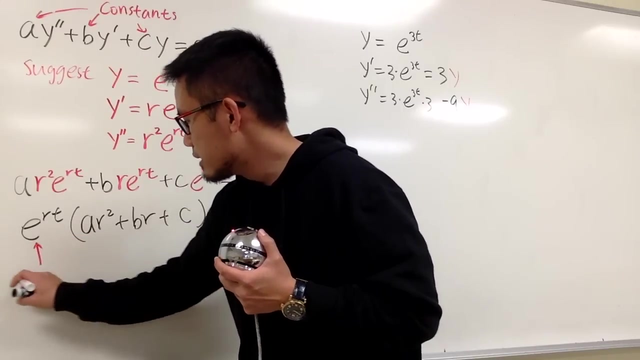 e to the rt, And that will give us: ar squared plus br plus c equals to zero. All right, this is an exponential part right. Exponential function e to the, something This right here we know is negative, Never zero, isn't it? 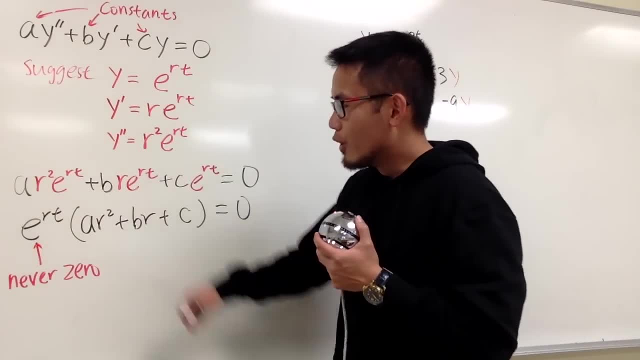 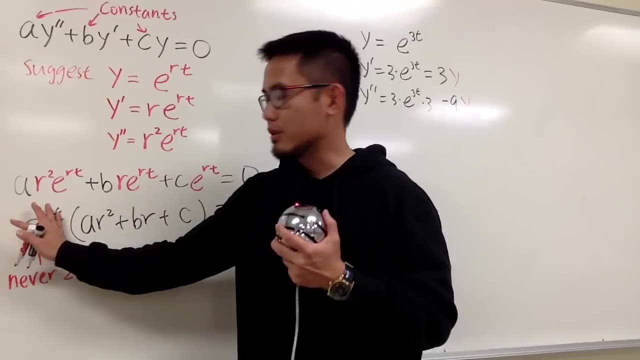 Never zero. let me just spell it out much better. So when we have this quantity, times that quantity, since e to the rt- is never zero. so you can either divide it out or you can just forget about it, because we just want to focus on this. 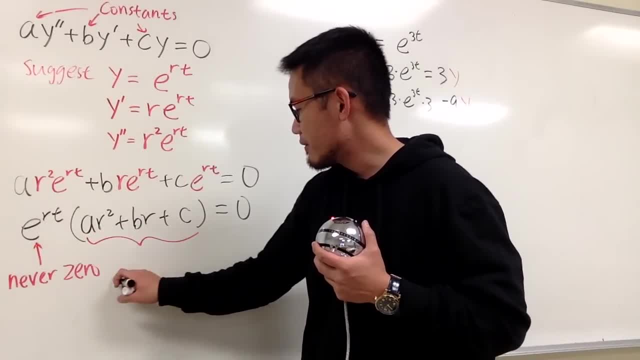 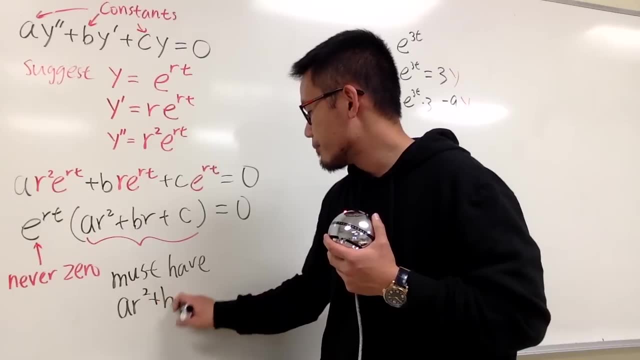 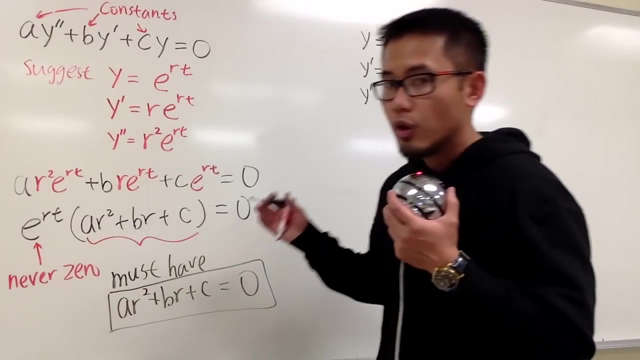 So that means we must have this part. We must have- let me just write it down- We must have the situation that ar squared plus br plus c, equal to zero. In fact, this, right here, is the condition that we need, Because from here this is pretty much just a quadratic equation, isn't it? 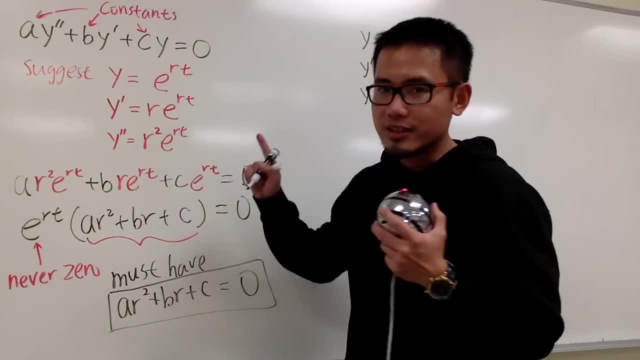 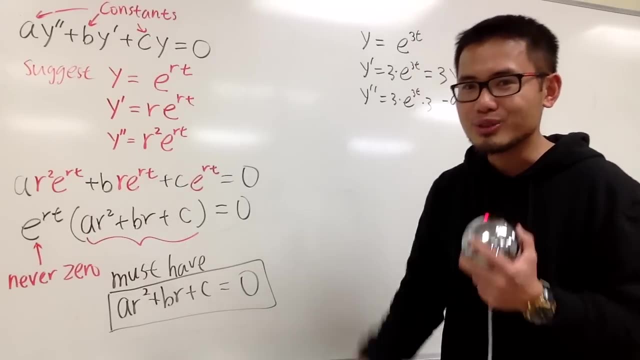 Quadratic equation in terms of r. From here we can solve for r and we can just plug it into the r here and we can generate the building blocks of the solution. And I'll show you guys what I mean by that. 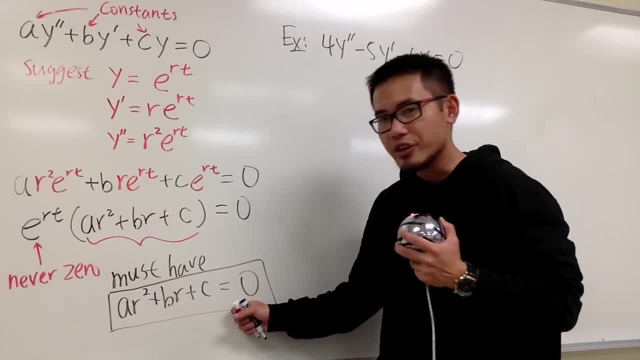 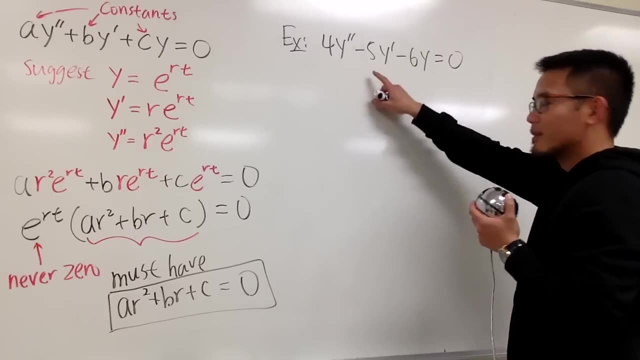 And before I show you guys an example, let me tell you guys that this equation here has a name. This is called the characteristic equation and this is also called the acceleration equation. And now let's go ahead and solve this, For y double prime minus 5y. prime minus 6y is equal to zero. 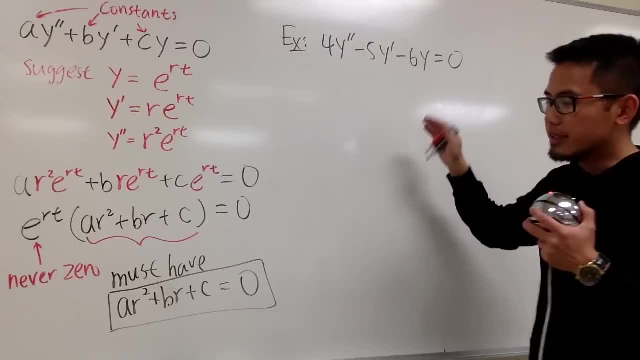 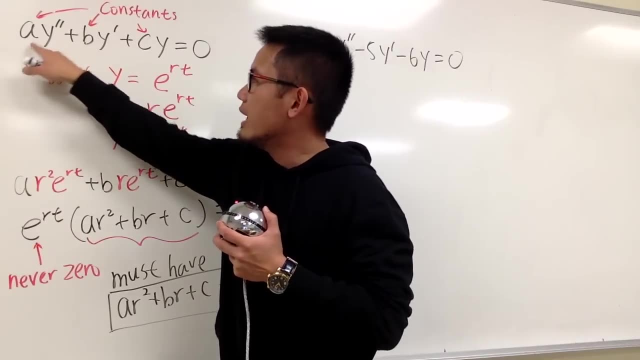 The first step is we have to take this and change it to its corresponding characteristic equation And check this out Earlier, when we started with ay double prime, we will end up ar squared right. So y double prime corresponds to r squared. 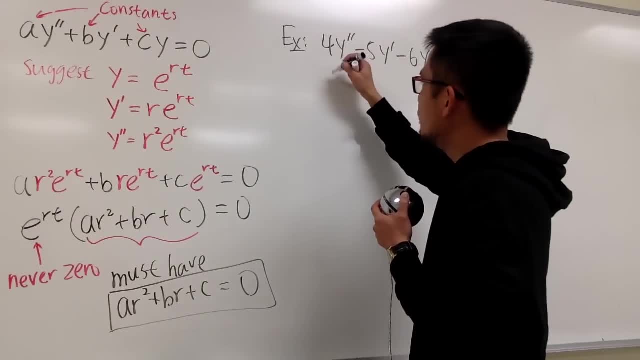 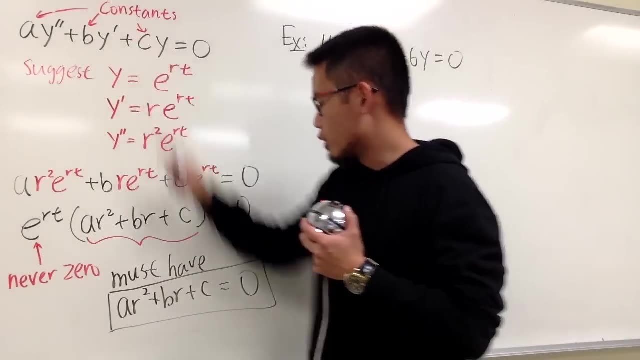 That means right here. the first term is going to give me 4.. So that's going to give me r squared. And then we just continue Minus 5, and the y prime corresponds with r. We change that to r, right here. 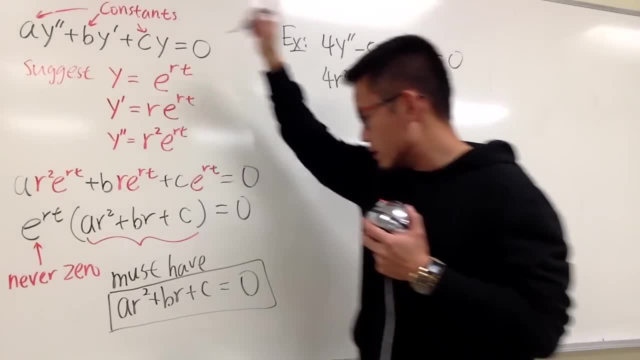 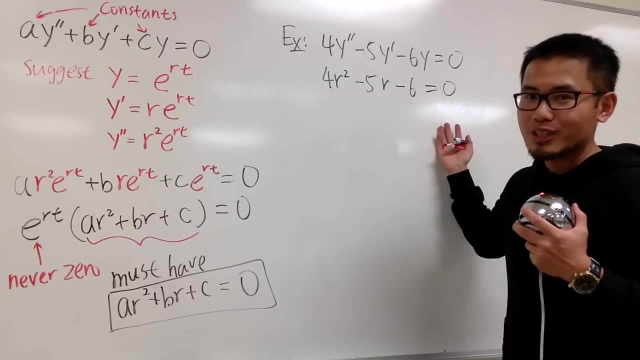 And then minus 6.. If you have y, we didn't have any r, right? So this is just minus 6.. This is it, And now we just have to solve this quadratic equation and do it whichever way that you would like. 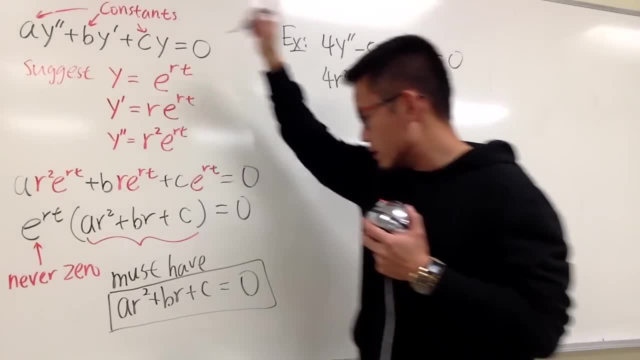 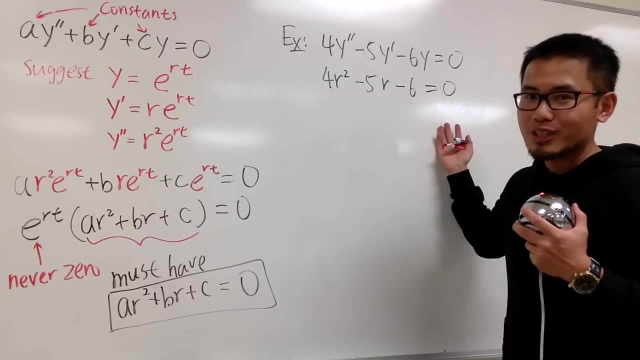 And then minus 6.. If you have y, we didn't have any r, right? So this is just minus 6.. This is it, And now we just have to solve this quadratic equation and do it whichever way that you would like. 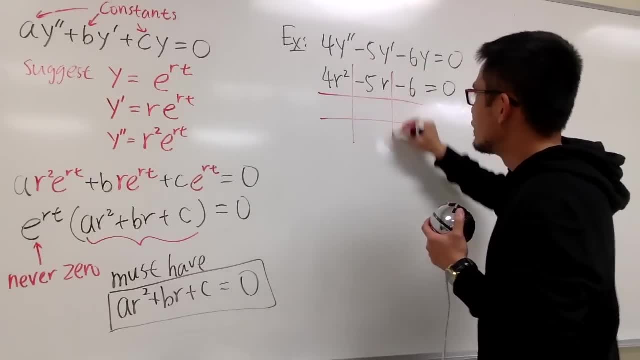 And I will factor this out for you guys And I'll show you guys with the tic-tac-toe factoring. And to do so I will have to ask myself what times 4 will give me 4r squared, And let me tell you guys the correct combination. 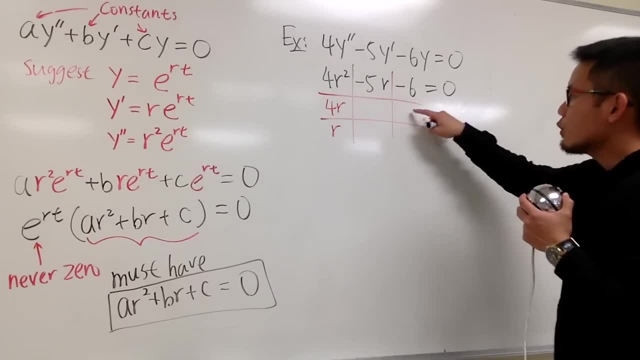 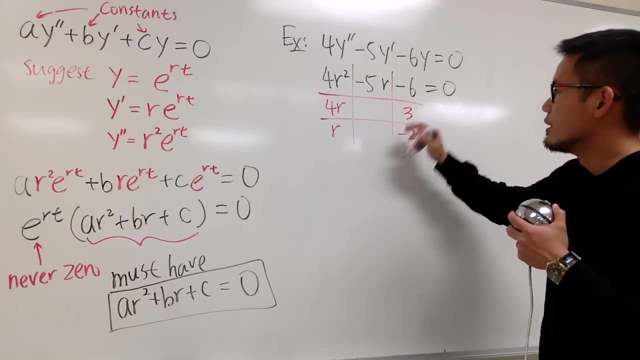 which is 4r times r, And what times 4 will give me negative 6?. And once again, let me tell you guys the correct combination, which is negative 2 plus 3, in these boxes like this, in this order: 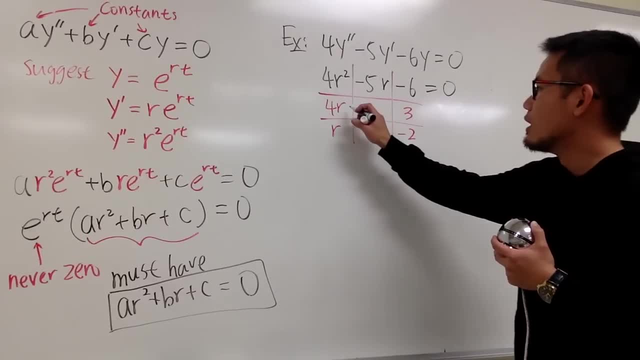 Well, I will convince you guys, this is correct To do so. you cross-multiply 4r times negative 2, which is negative 8r, And then you take 3 times r, which is 3r. It is correct, because negative 8r plus 3r is negative 5r. 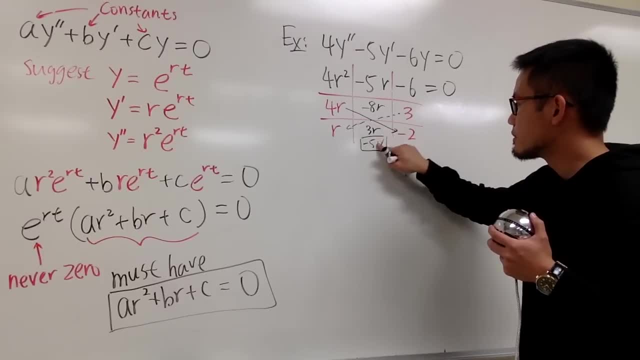 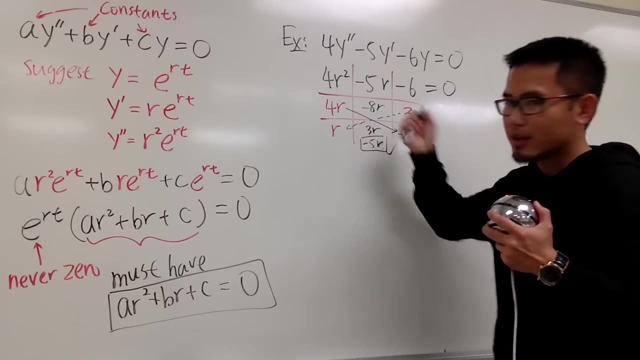 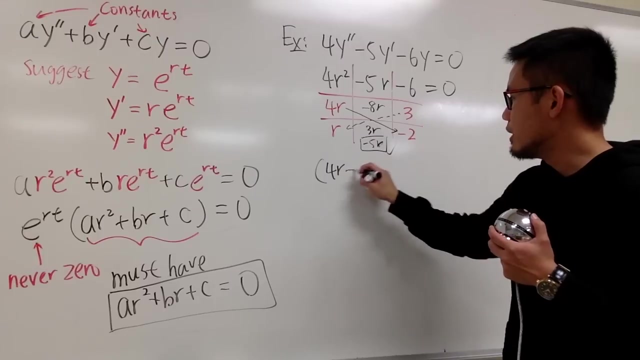 So this is correct, isn't it Right? Okay, so that's good, And now we have to read the answers correctly from the boxes here, To read the answers you go across. So the first factor is going to be 4r plus 3.. 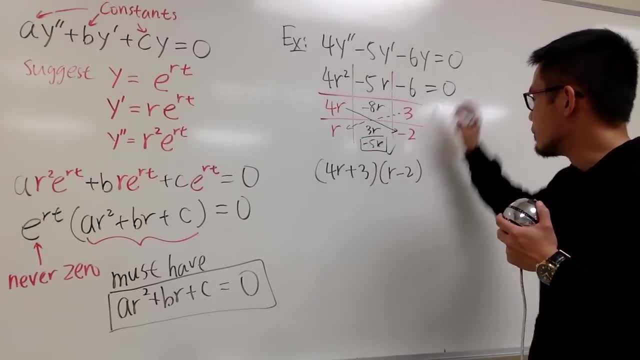 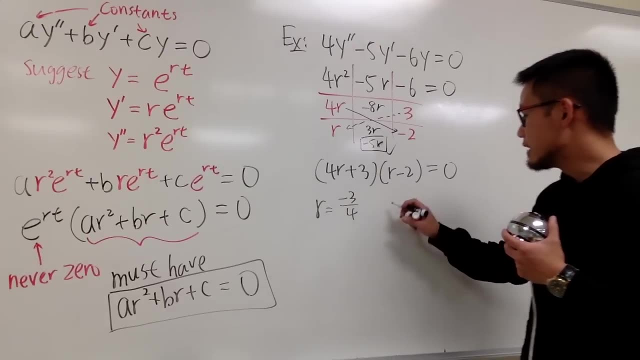 And the second one is r minus 2.. And we still have equal to 0,, of course, Alright. for the first one, we know, r is equal to negative 3 over 4.. And for the second one, we know, r is equal to 2.. 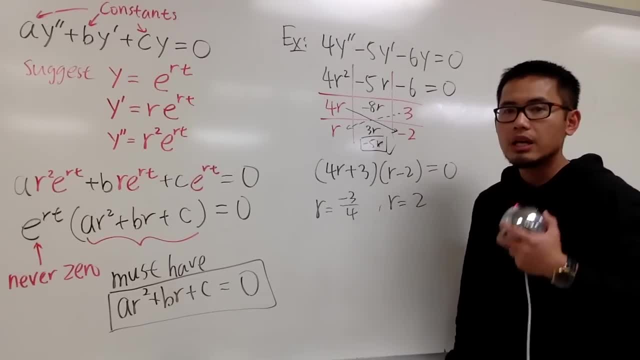 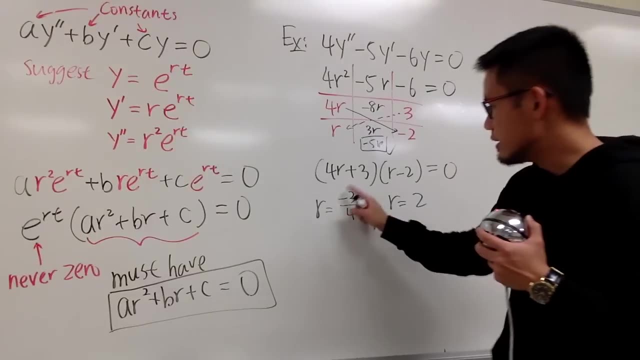 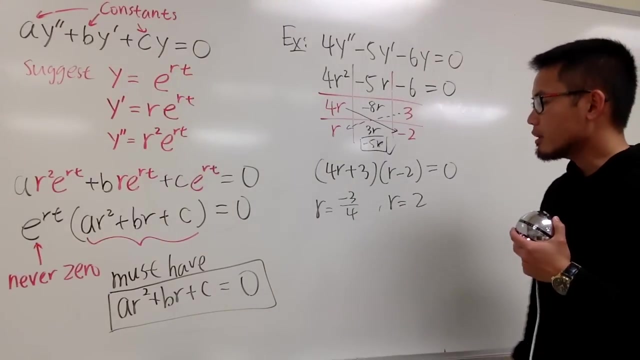 And you see, we end up with two different r values. In this case, we will end up with two different building blocks for the solution: e to the first r, which is this, and then times t. The second one is going to be e to the 2t right. 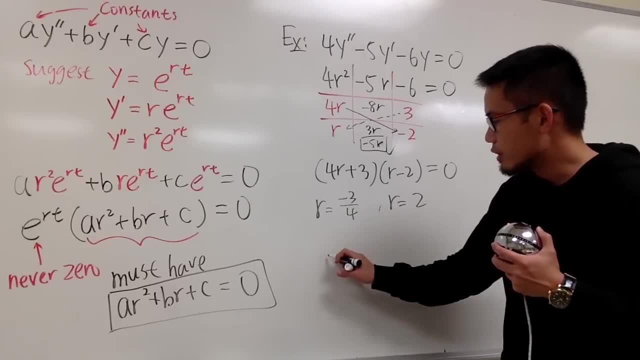 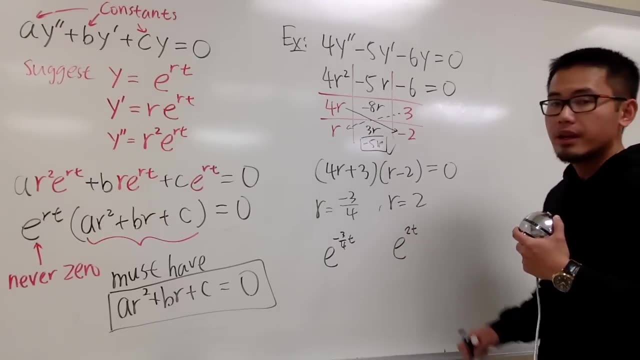 So let me just write down the building blocks for you guys. first, This right here is going to give me e to the negative 3 over 4t, And the second one is going to give me e to the 2t, And I'm going to explain to you guys. 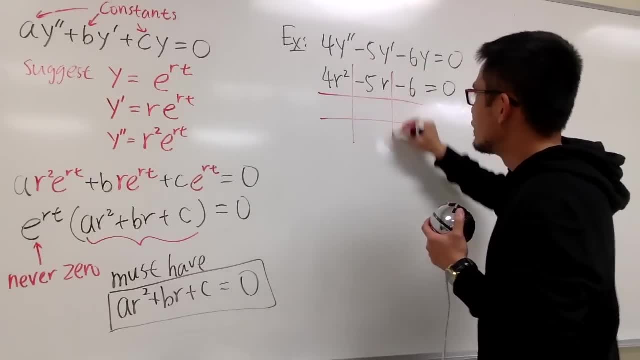 And I will factor this out for you guys And I'll show you guys with the tic-tac-toe factoring. And to do so I will have to ask myself what times 4 will give me 4r squared, And let me tell you guys the correct combination. 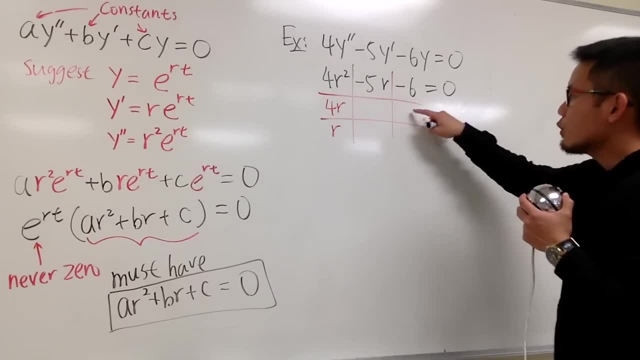 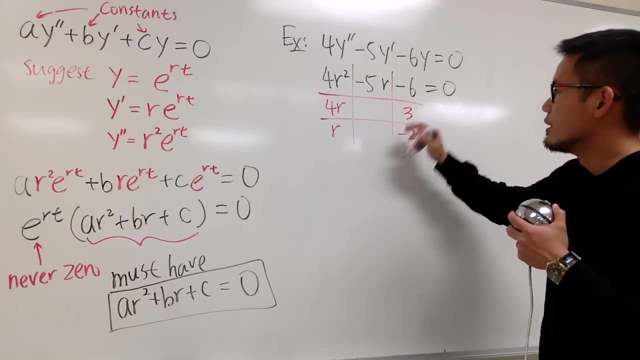 which is 4r times r, And what times 4 will give me negative 6?. And once again, let me tell you guys the correct combination, which is negative 2 plus 3, in these boxes like this, in this order: 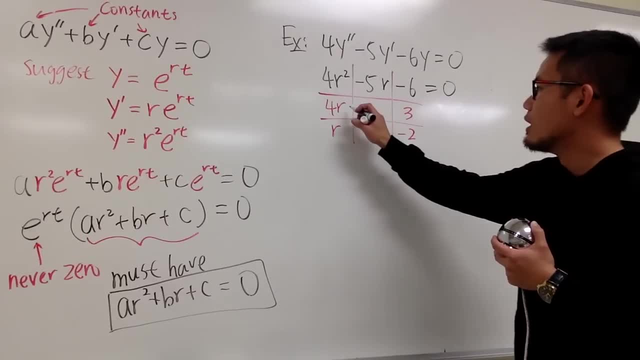 Well, I will convince you guys, this is correct To do so. you cross-multiply 4r times negative 2, which is negative 8r, And then you take 3 times r, which is 3r. It is correct, because negative 8r plus 3r is negative 5r. 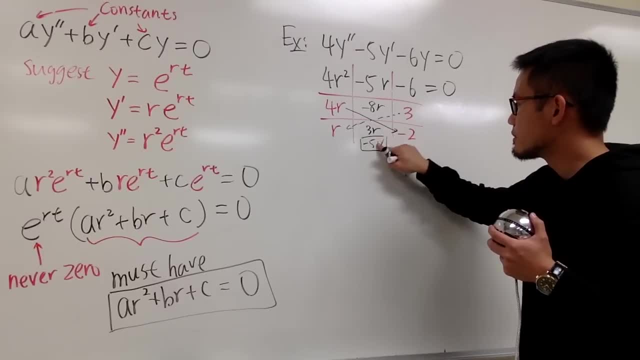 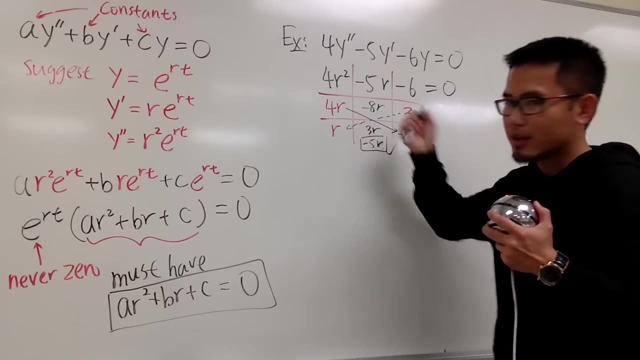 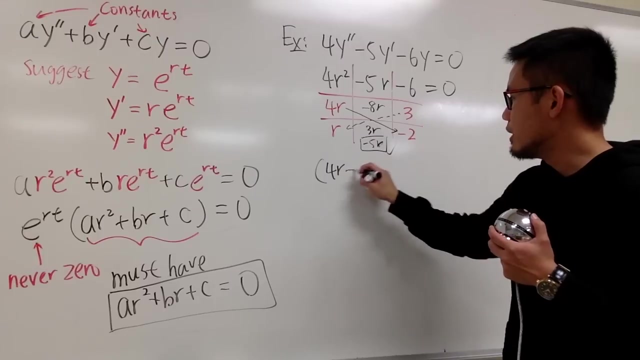 So this is correct, isn't it Right? Okay, so that's good, And now we have to read the answers correctly from the boxes here, To read the answers you go across. So the first factor is going to be 4r plus 3.. 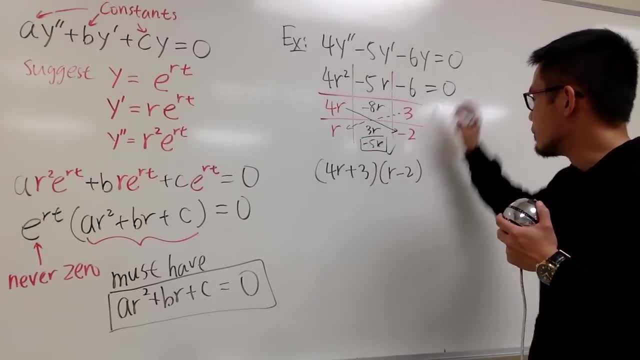 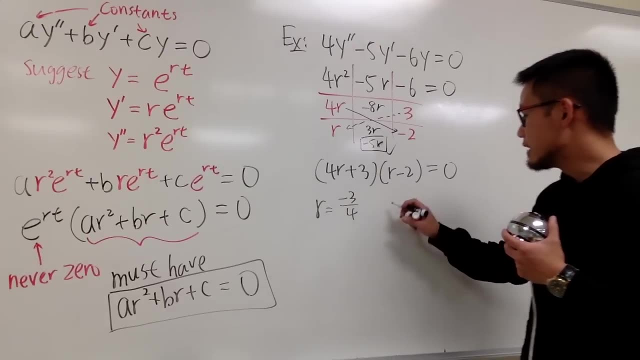 And the second one is r minus 2.. And we still have equal to 0,, of course, Alright. for the first one, we know, r is equal to negative 3 over 4.. And for the second one, we know, r is equal to 2.. 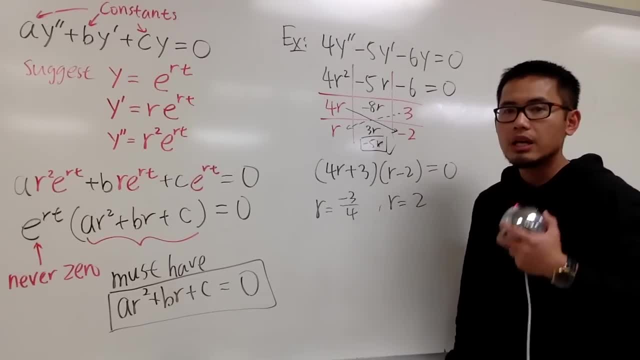 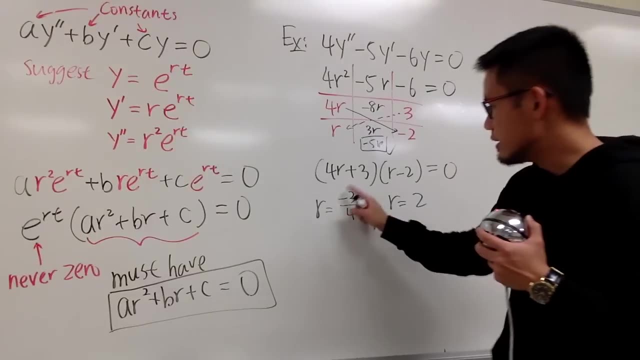 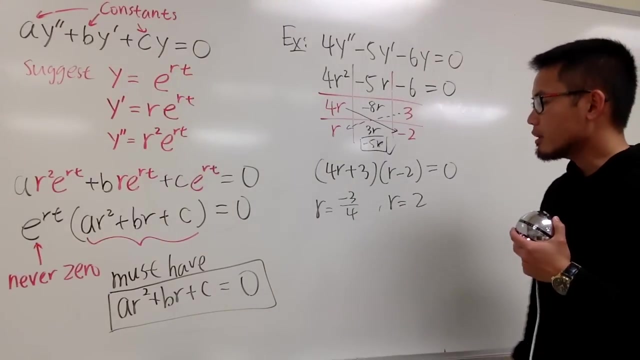 And you see, we end up with two different r values. In this case, we will end up with two different building blocks for the solution: e to the first r, which is this, and then times t. The second one is going to be e to the 2t right. 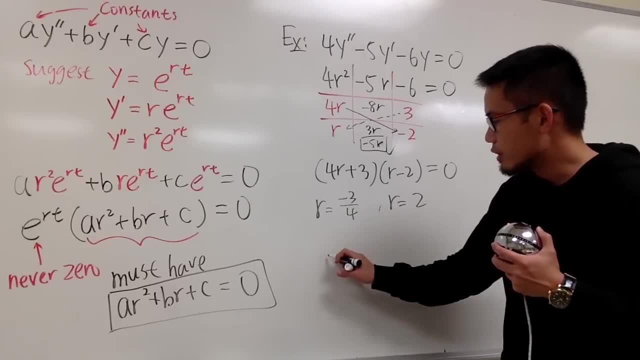 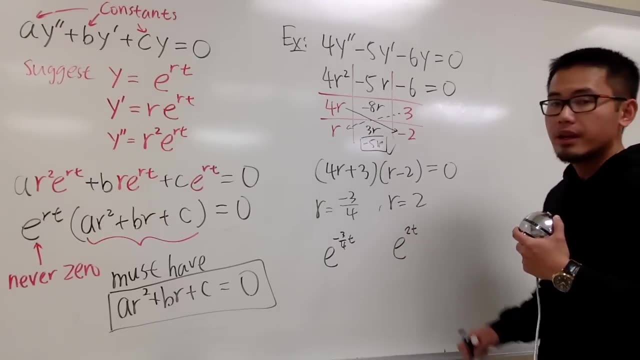 So let me just write down the building blocks for you guys. first, This right here is going to give me e to the negative 3 over 4t, And the second one is going to give me e to the 2t, And I'm going to explain to you guys. 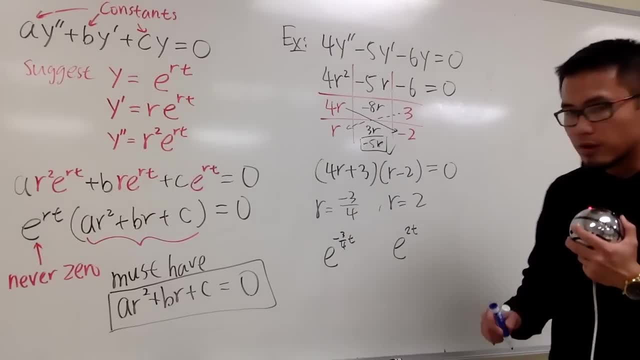 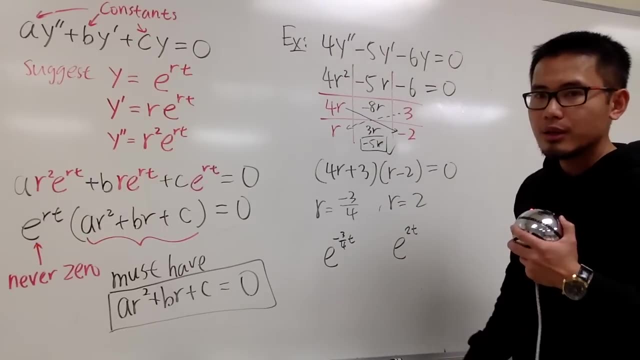 what do I mean by building blocks? First of all, let me just show you guys that both of them will satisfy the original differential equation And just for simplicity purpose, let me just check this one for you guys only. okay, And you can do this on your own. 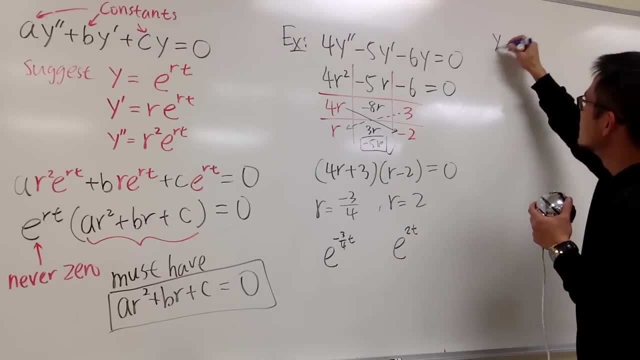 So let me just put down this right here. Let me just say this is the second one, I guess. So let me put down y2.. y2 equals to e, to the 2t, And then what I have to do is differentiate this. 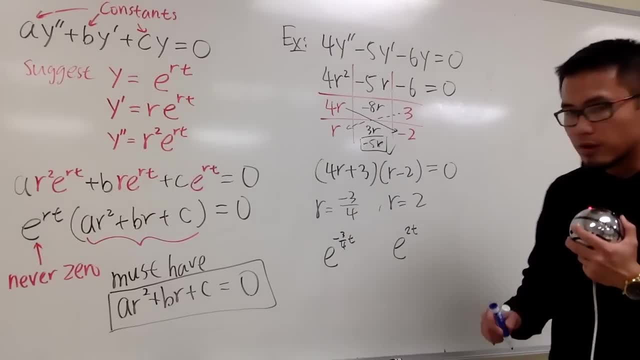 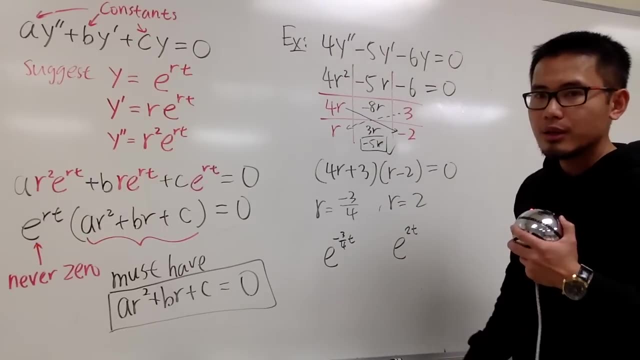 what do I mean by building blocks? First of all, let me just show you guys that both of them will satisfy the original differential equation And just for simplicity purpose, let me just check this one for you guys only. okay, And you can do this on your own. 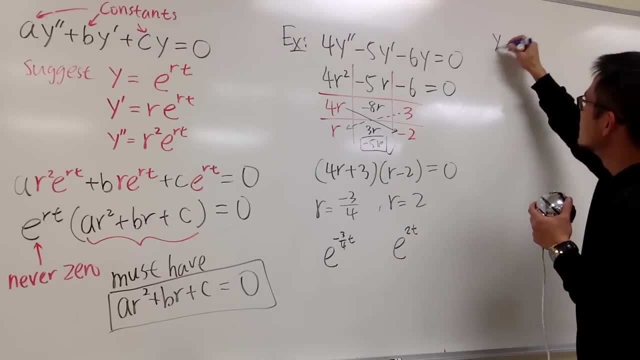 So let me just put down this right here. Let me just say this is the second one, I guess. So let me put down y2.. y2 equals to e, to the 2t, And then what I have to do is differentiate this. 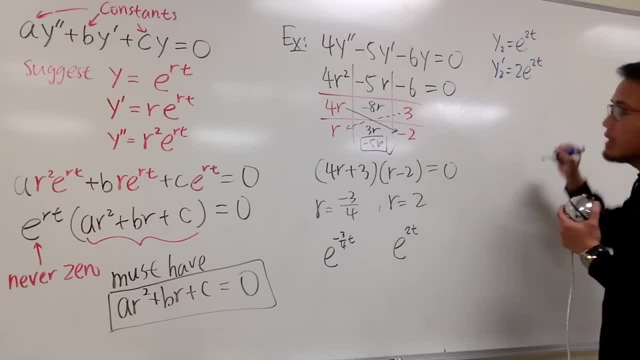 which is going to give me 2e2t right. And then I'll do it again: y2 double prime, which is 4e2t right. And now I will plug in all this into the original And you see it will give me 4, right. 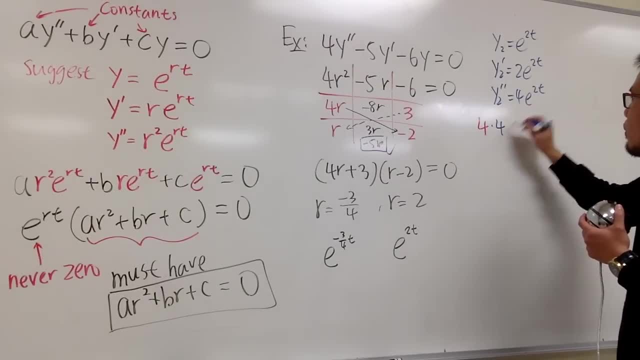 And y double prime, which is that: So we multiply by 4e2t And then minus 5. y, prime, which is that which is times 2e2t And then minus 6. y, which is that. 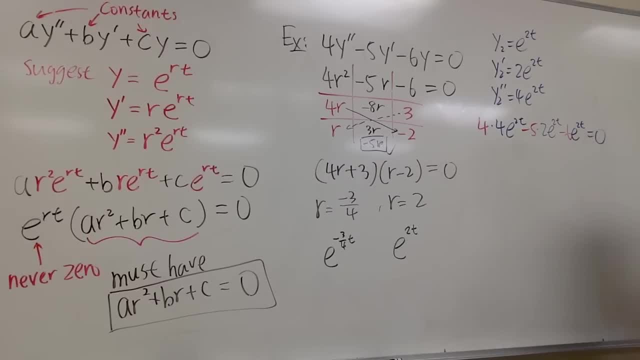 e to the 2t. like this: Do we end up with 0? Yes, we do. This is 16.. Minus 10,, which is 6. And then minus 6.. Of course, everything ends up to be 0.. 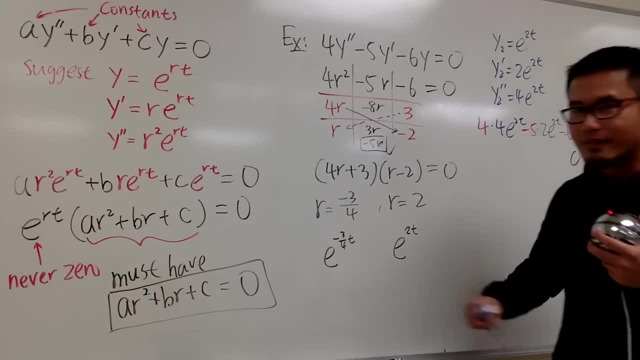 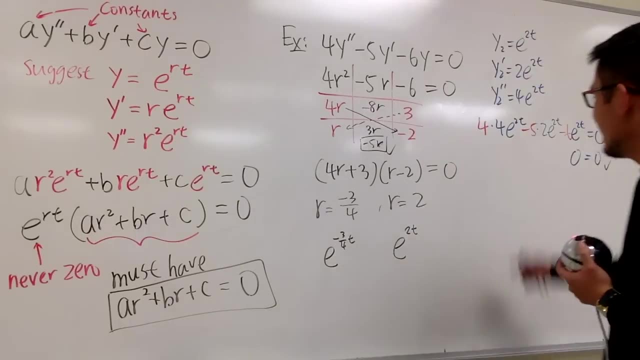 So 0 is equal to 0. So it checks This right here. This right here definitely works, isn't it? And you can do exactly the same thing for this, but you can also take my word for it, It will work out nicely as well. 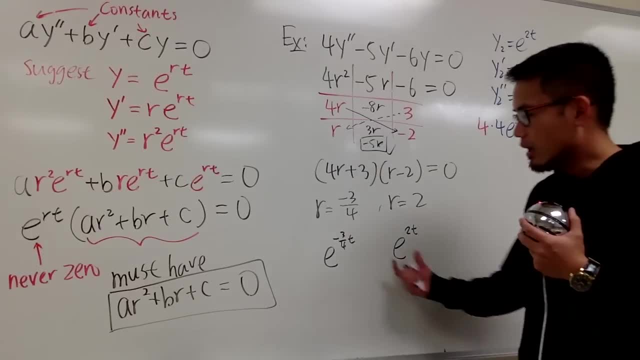 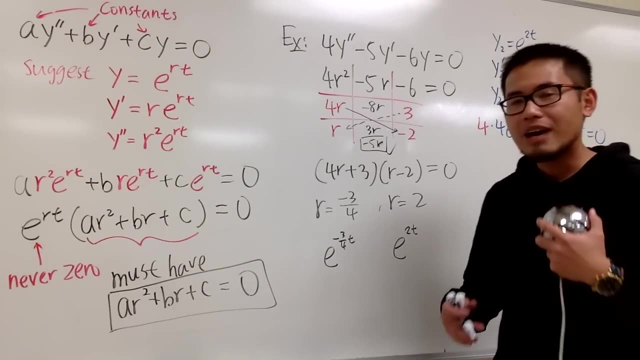 All right Now. these are just the function part. What we'll be doing is that? well, remember, when we're solving differential equations we have that constant right And keep in mind whenever we have the second-order differential equation. 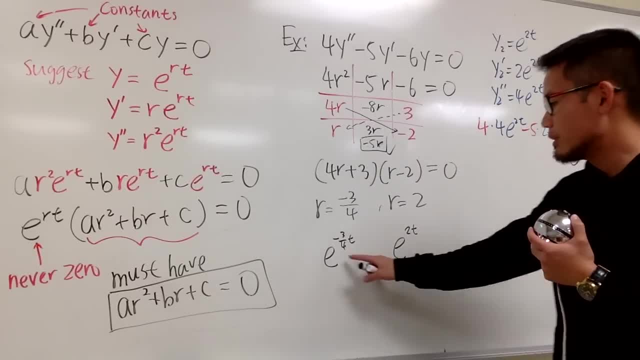 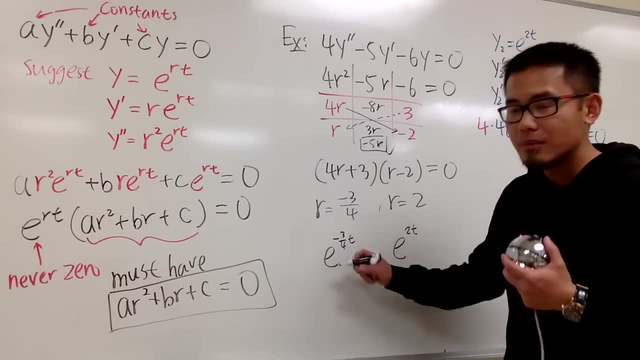 we will have two different constants. Well, do I put down plus c or divide by c? I don't know. The truth is, we multiply the function part by c1 and c2.. So this right here is c1,. 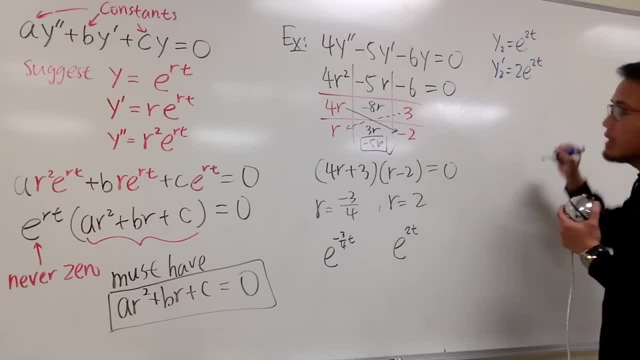 which is going to give me 2e2t right. And then I'll do it again: y2 double prime, which is 4e2t right. And now I will plug in all this into the original And you see it will give me 4, right. 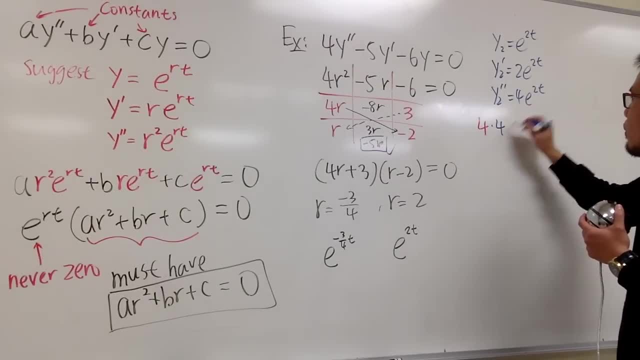 And y double prime, which is that: So we multiply by 4e2t And then minus 5. y, prime, which is that which is times 2e2t And then minus 6. y, which is that. 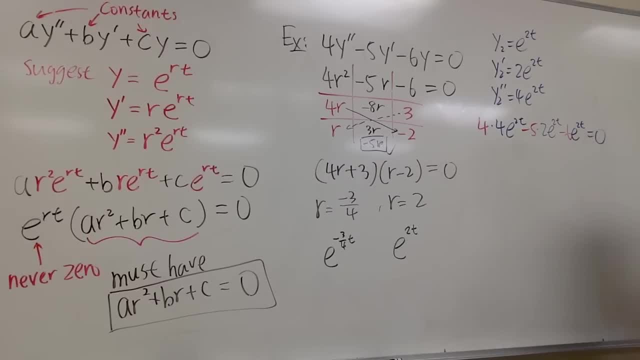 e to the 2t. like this: Do we end up with 0? Yes, we do. This is 16.. Minus 10,, which is 6. And then minus 6.. Of course, everything ends up to be 0.. 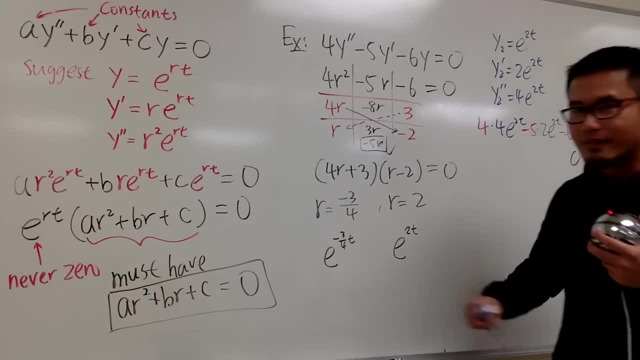 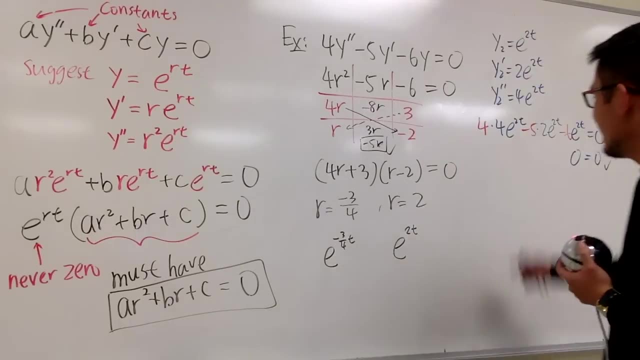 So 0 is equal to 0. So it checks This right here. This right here definitely works, isn't it? And you can do exactly the same thing for this, but you can also take my word for it, It will work out nicely as well. 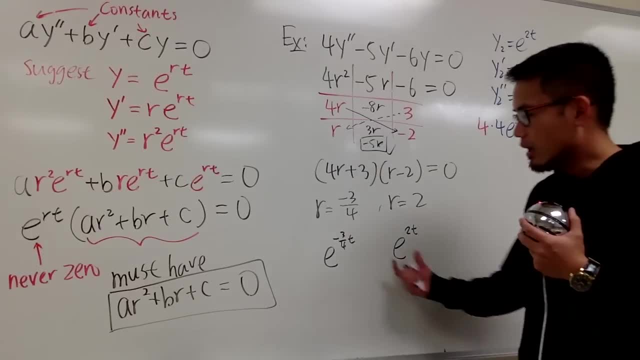 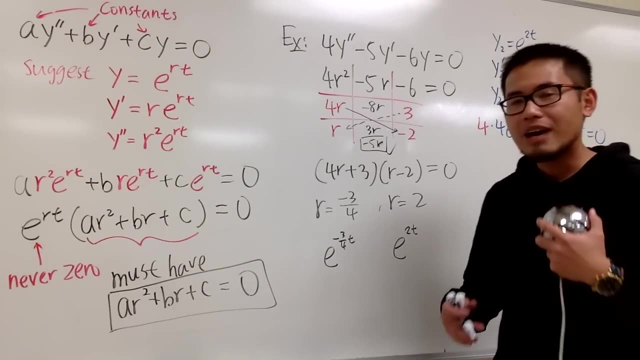 All right Now. these are just the function part. What we'll be doing is that? well, remember, when we're solving differential equations we have that constant right And keep in mind whenever we have the second-order differential equation. 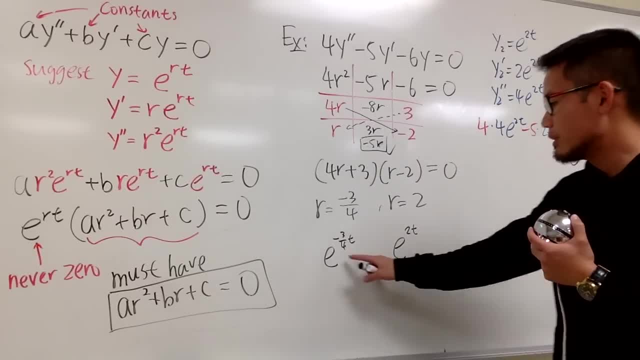 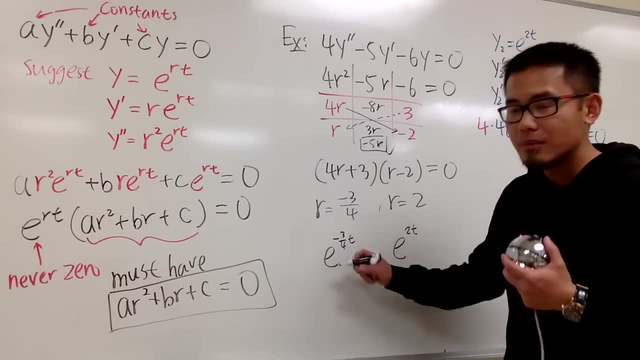 we will have two different constants. Well, do I put down plus c or divide by c? I don't know. The truth is, we multiply the function part by c1 and c2.. So this right here is c1,. 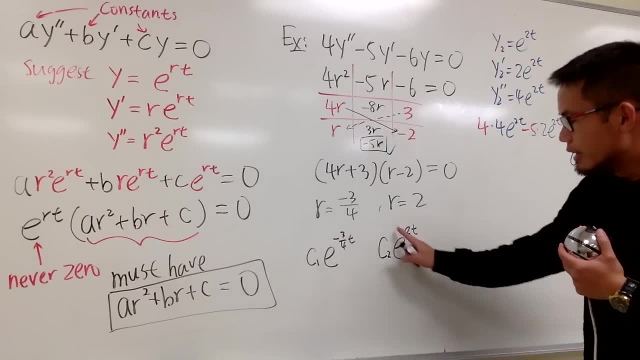 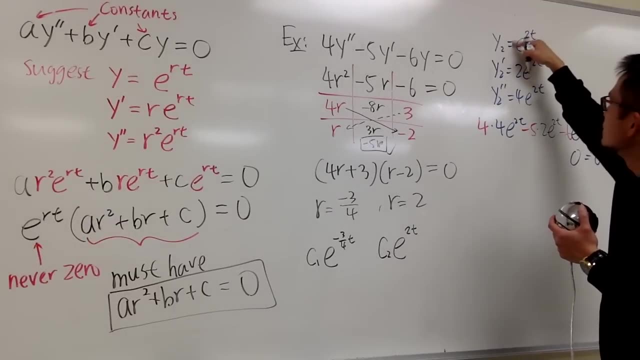 and this right here is c2.. So let me just demonstrate this right here on the side for you guys real quick, Because now you see when I multiply this function by c, so let me just put down c in black like this: 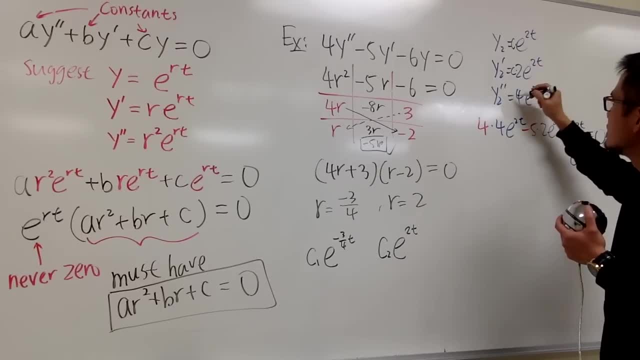 Guess what? I will just have to multiply everything by c, isn't it c and c? And then pretty much this term. we'll now have a c right here, and this function here, this part here, has a c here as well. 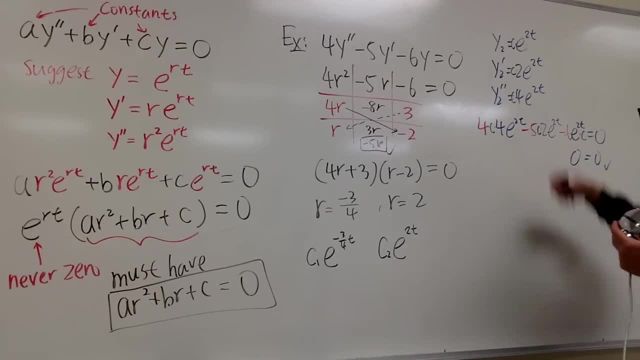 This right here. just multiply by c, right, We're just plugging everything accordingly. Guess what, When I have this c here, I will still end up with 0. on the left-hand side, Of course, still equals 0.. 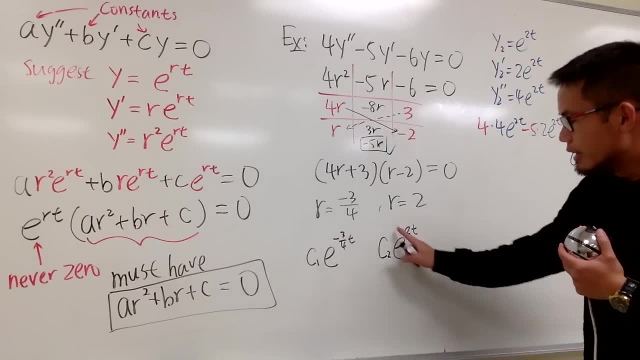 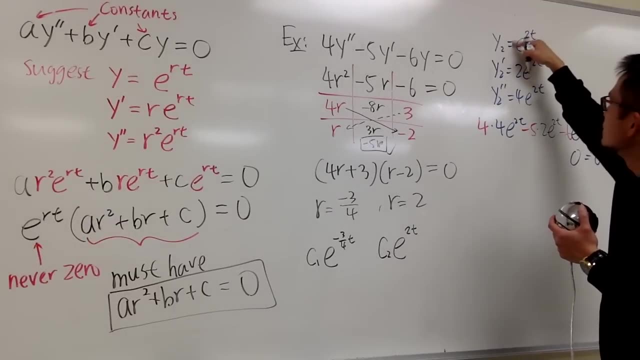 and this right here is c2.. So let me just demonstrate this right here on the side for you guys real quick, Because now you see when I multiply this function by c, so let me just put down c in black like this: 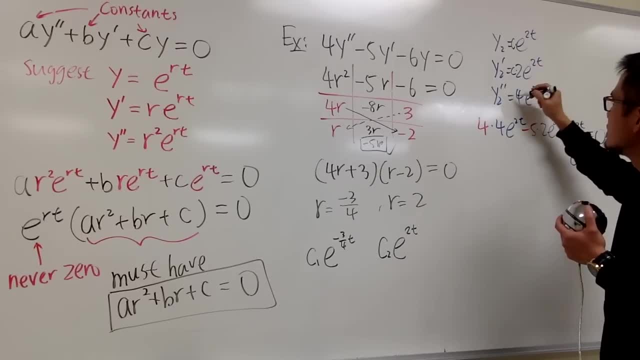 Guess what? I will just have to multiply everything by c, isn't it c and c? And then pretty much this term. we'll now have a c right here, and this function here, this part here, has a c here as well. 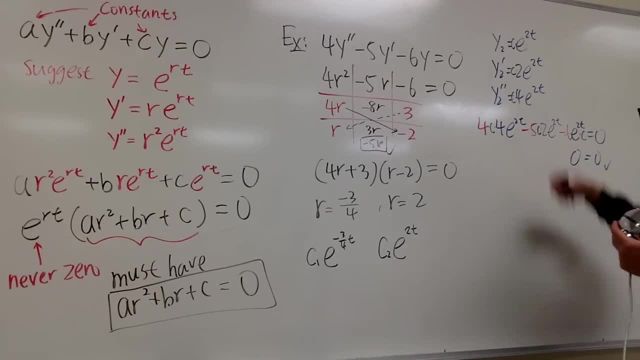 This right here. just multiply by c, right, We're just plugging everything accordingly. Guess what, When I have this c here, I will still end up with 0. on the left-hand side, Of course, still equals 0.. 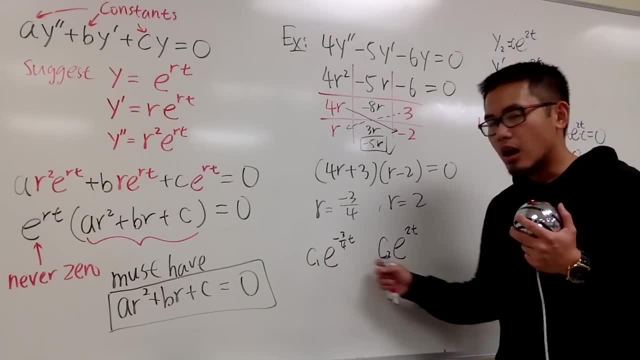 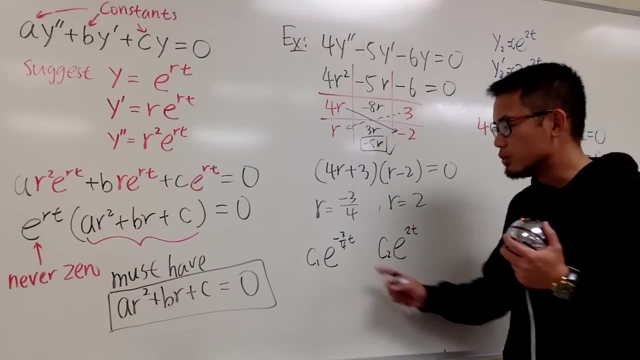 The point of that is to show you these are the places where c should be. c1 and c2 are just the multiple of the function part. c1 and c2 are just the multiple of the building blocks of the solutions At the end. 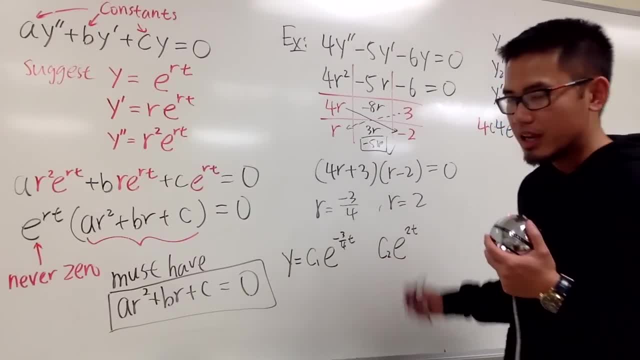 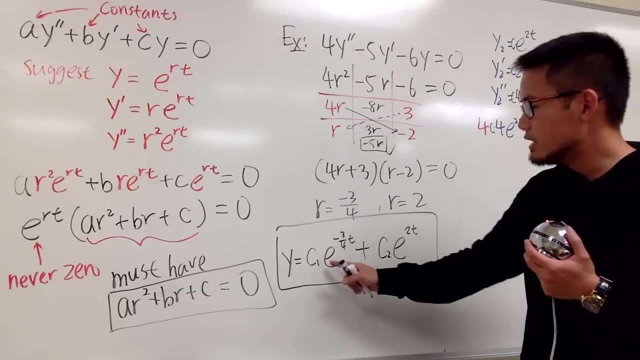 the overall solution is that you are just going to add them together, and this is it. This is the solution for that. y is equal to c1, e to the negative 0 for t, plus c2 e to the 2t. That's it. 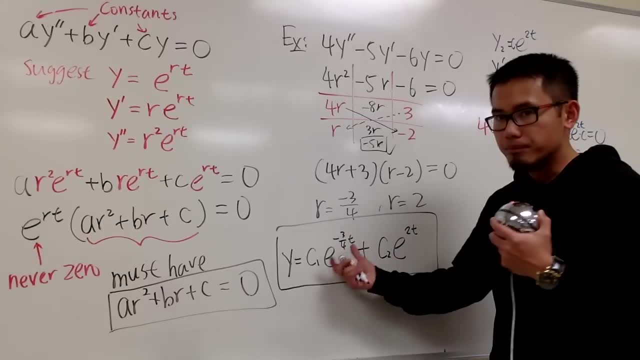 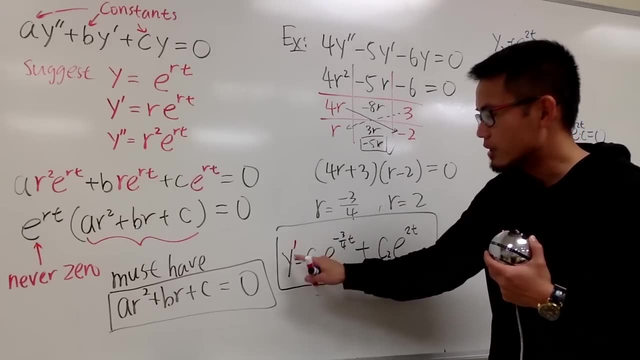 And the truth is that we can just add them together and this is the overall solution. It's because when you differentiate this right, Imagine if I'm differentiating the y- Well, I just have to differentiate the first and the second is that 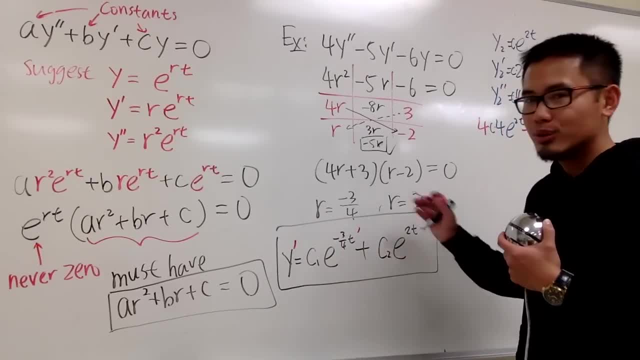 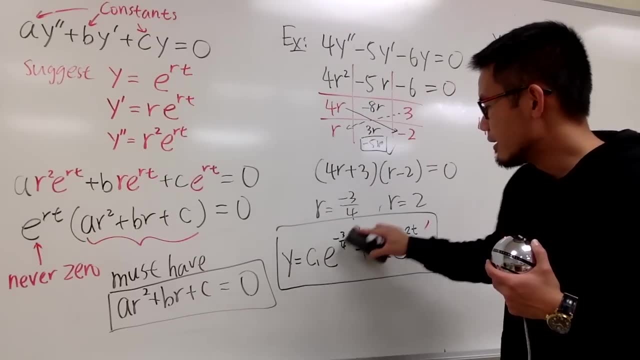 differentiate this and differentiate that, Do it again, do it again, do it again. Plug in, plug in, plug in. You get 0 is equal to 0 once again. So this is the idea. Just to summarize this real quick. 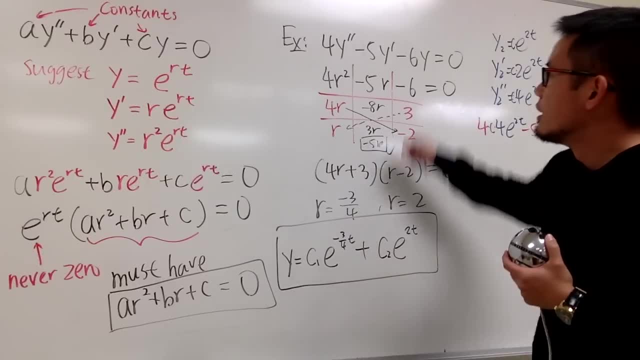 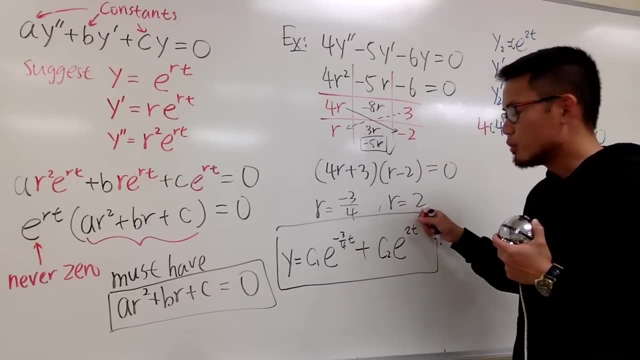 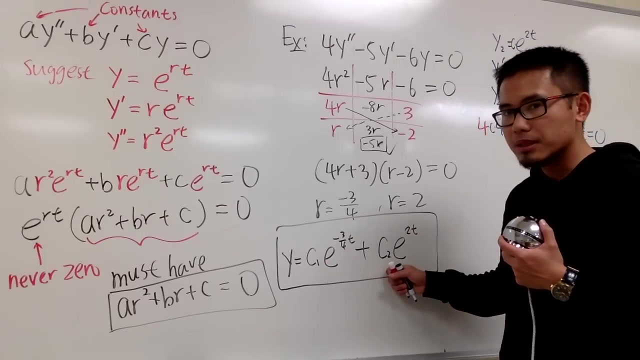 All you have to do just to keep everything simple: get the characteristic equation, solve the quadratic equation in R. if you get two different R values, well, e to the first, R times t e to the second, R plus t, and be sure you multiply c1 and c2 correspondingly. 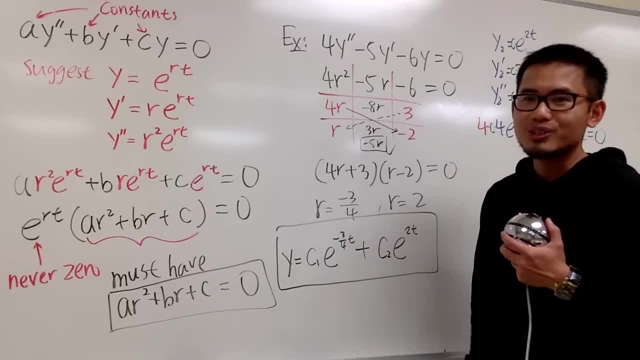 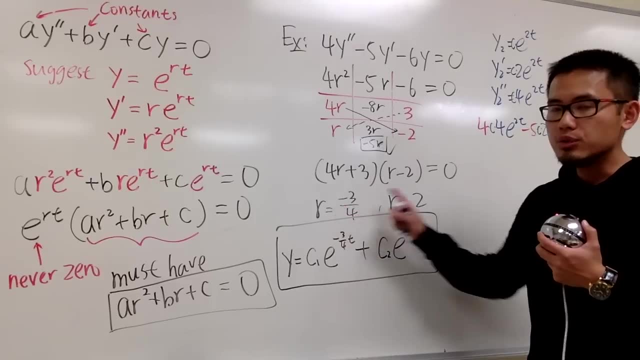 and then add them together. This is the general solution. This is the first situation. You should watch my next video. I will show you what happens when I have these two R values being the same. 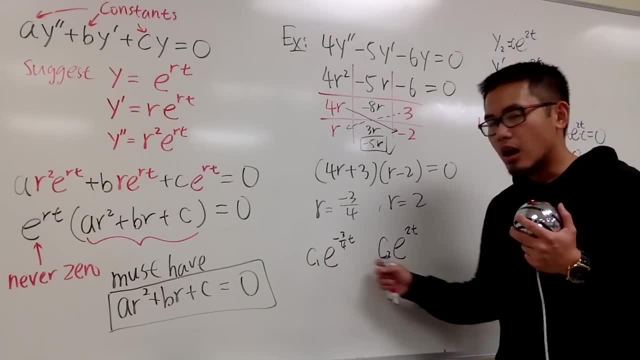 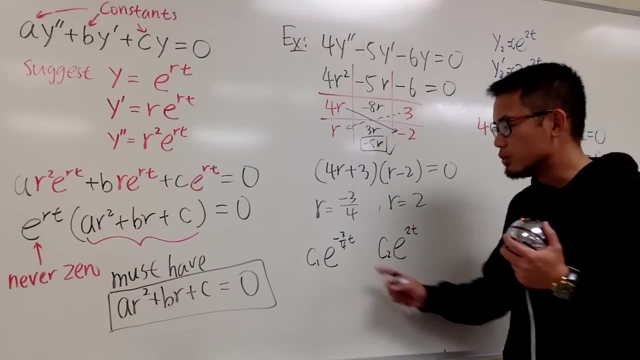 The point of that is to show you these are the places where c should be. c1 and c2 are just the multiple of the function part. c1 and c2 are just the multiple of the building blocks of the solutions At the end. 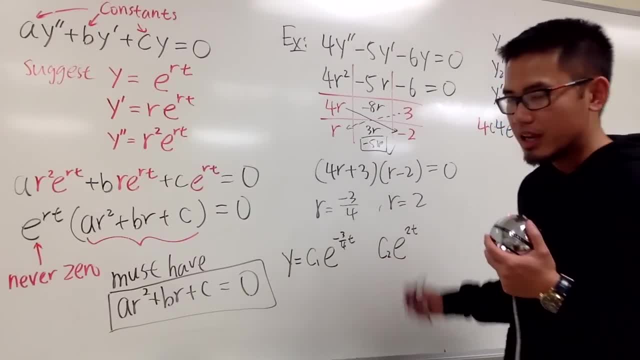 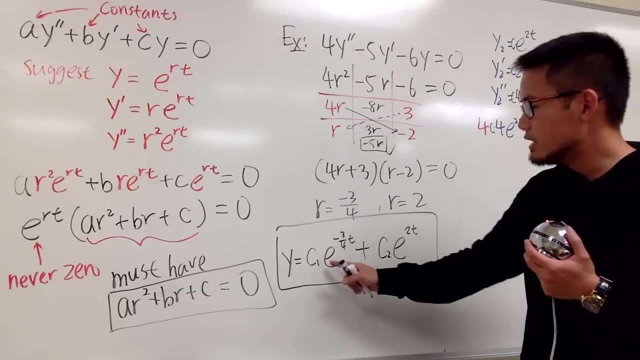 the overall solution is that you are just going to add them together, and this is it. This is the solution for that. y is equal to c1, e to the negative 0 for t, plus c2 e to the 2t. That's it. 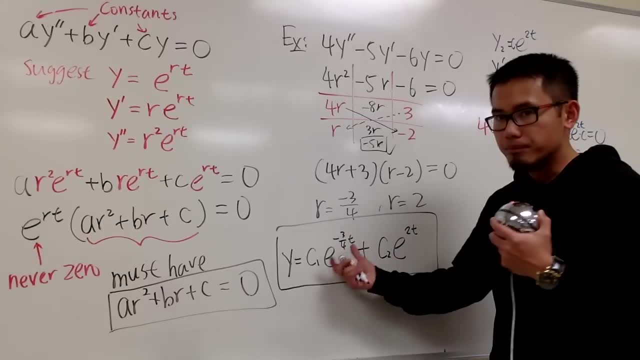 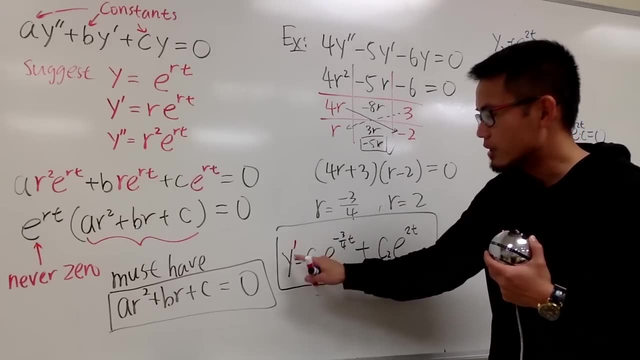 And the truth is that we can just add them together and this is the overall solution. It's because when you differentiate this right, Imagine if I'm differentiating the y- Well, I just have to differentiate the first and the second is that 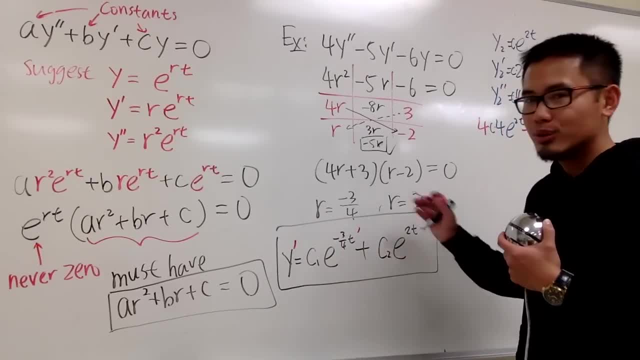 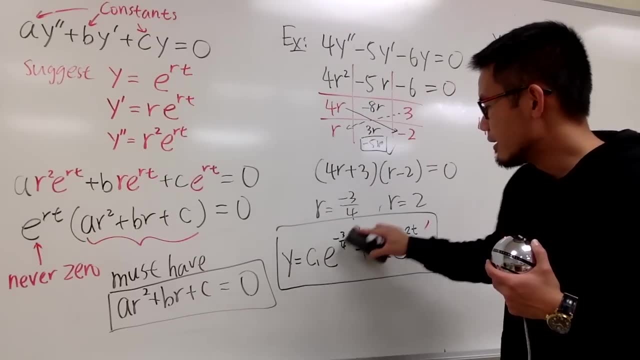 differentiate this and differentiate that, Do it again, do it again, do it again. Plug in, plug in, plug in. You get 0 is equal to 0 once again. So this is the idea. Just to summarize this real quick. 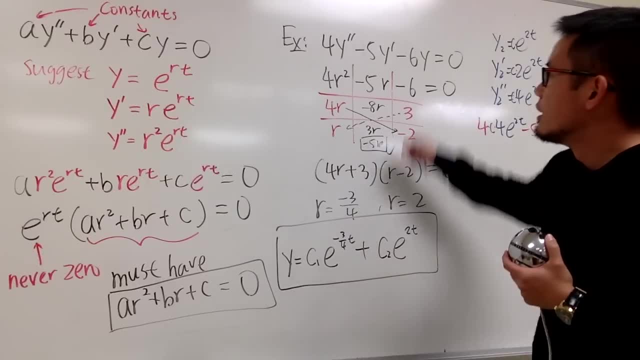 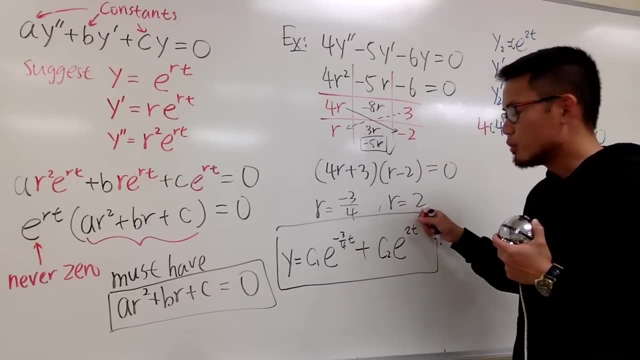 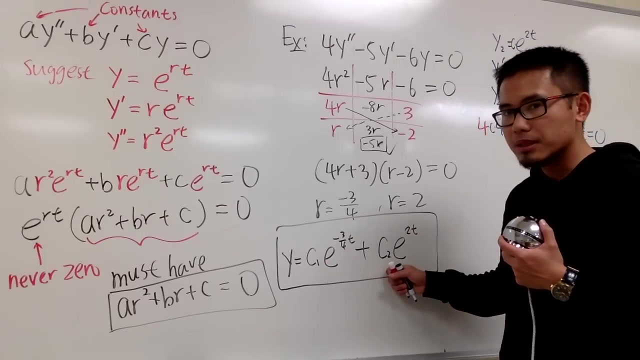 All you have to do just to keep everything simple: get the characteristic equation, solve the quadratic equation in R. if you get two different R values, well, e to the first, R times t e to the second, R plus t, and be sure you multiply c1 and c2 correspondingly. 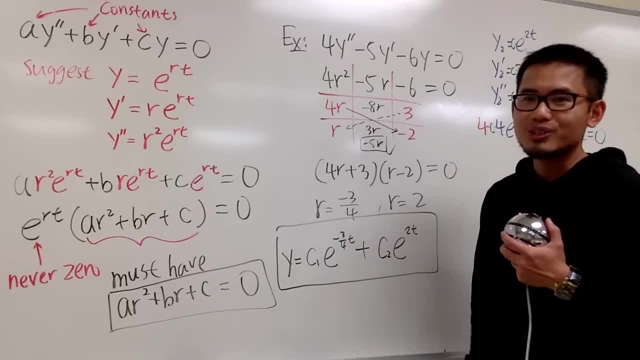 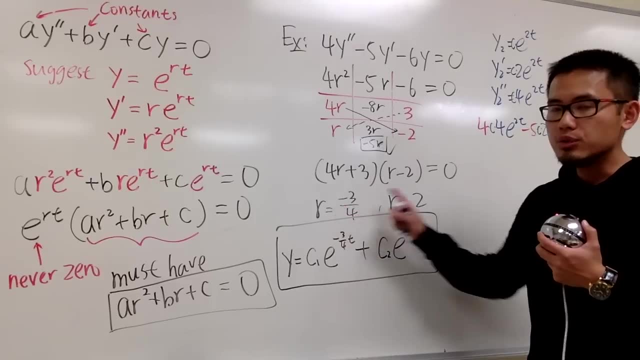 and then add them together. This is the general solution. This is the first situation. You should watch my next video. I will show you what happens when I have these two R values being the same. 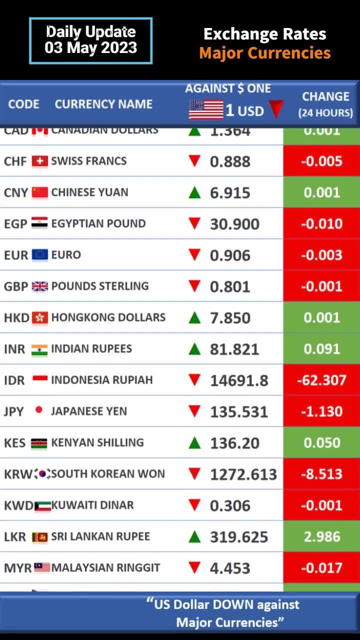 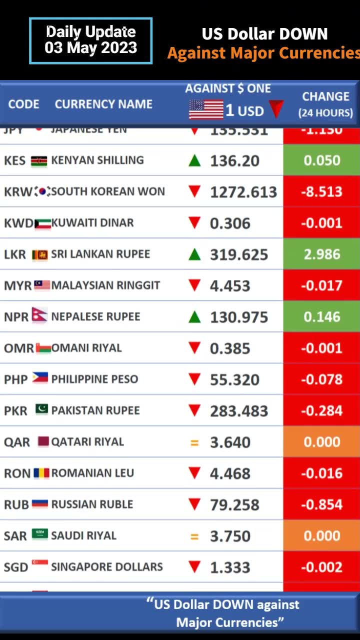 Please add punctuation in the appropriate places.